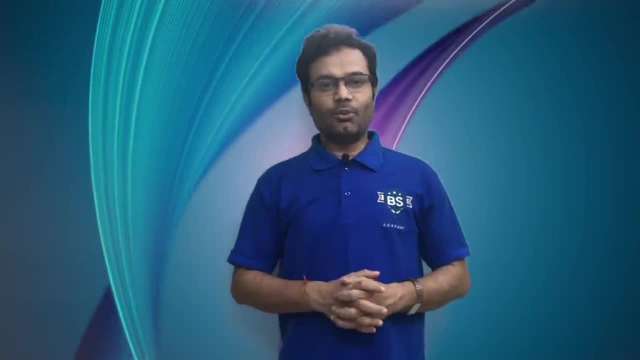 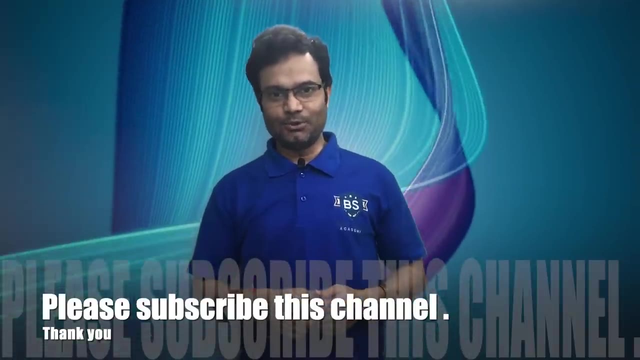 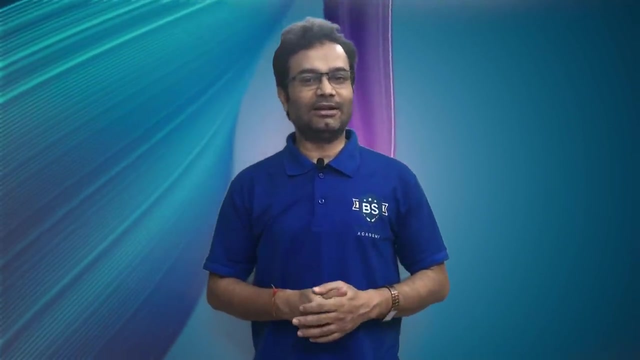 explain why these building blocks are very important, what is the mathematics behind that, how it is going to reduce the dimensionality of image or any input and how it is going to change the shape of input and what is the formula behind that. So I will explain everything in. 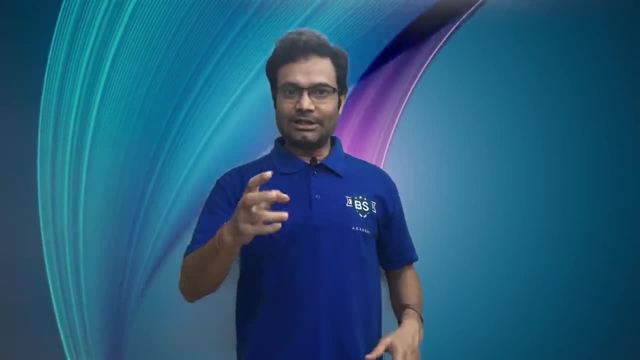 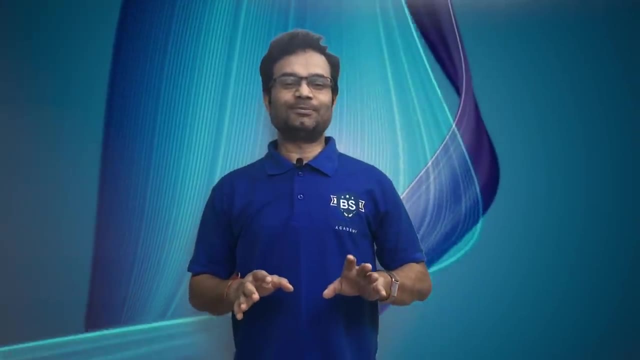 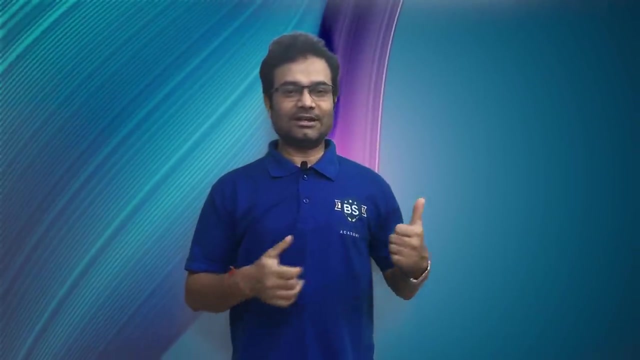 whiteboard to give more detail. each and everything I will explain and next video I will show everything through the code. I will be using the Keras TensorFlow to use all the concepts in the Jupyter Notebook. So let us start on the whiteboard. So this is the typical diagram of a 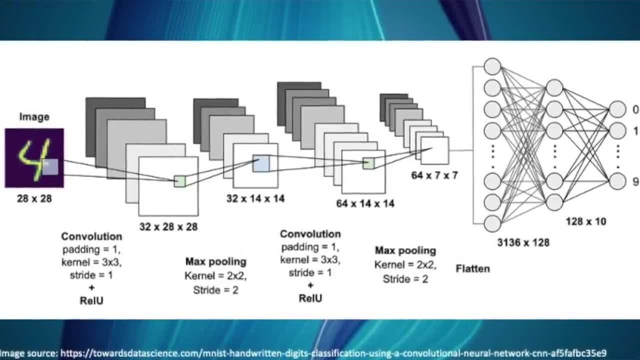 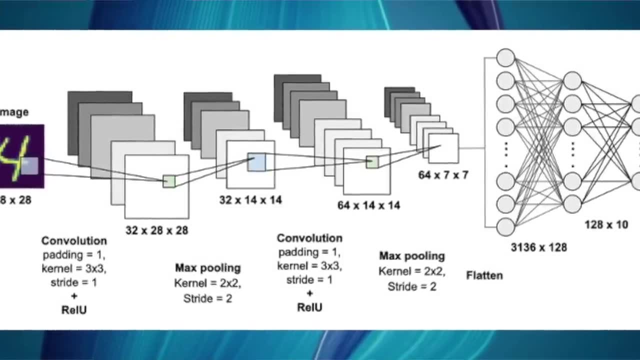 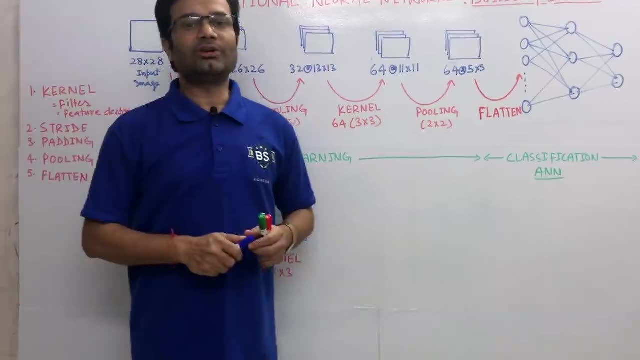 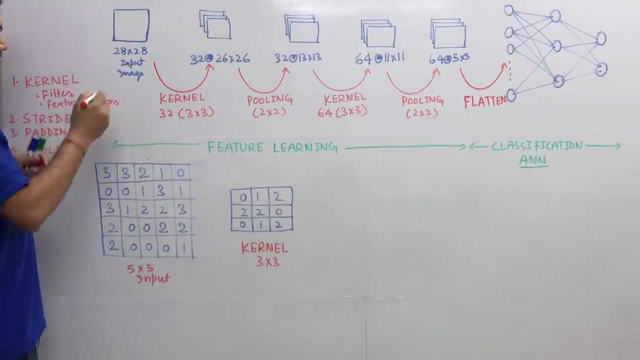 Conversion Neural Network and Conversion Neural Network is a category of Neural Network or deep learning that has proven very effectively in areas like image recognition, audio video recognition and their classification. If you see, this is our input image and this input image. we use the different kind of building blocks, like the: 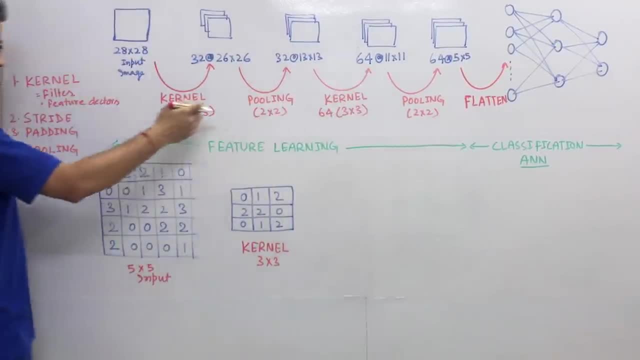 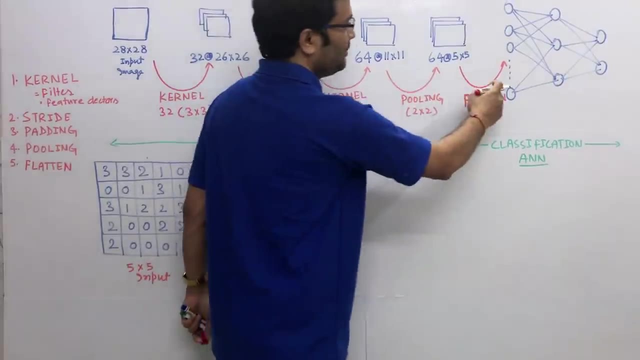 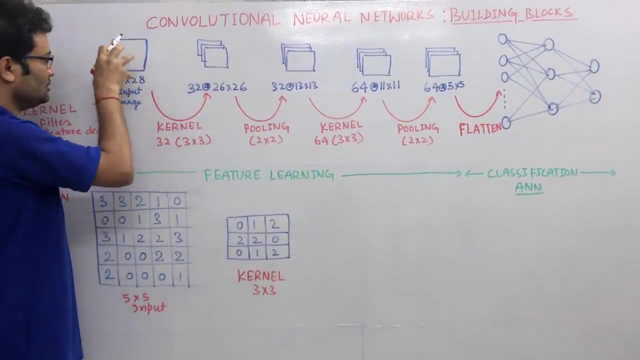 kernel pooling, then kernel, then this kind of stride padding pooling pattern and finally we reduce the dimensionality and pass into the fully connected network. But the question is that why I cannot use this image directly here, why I am going to reduce the. 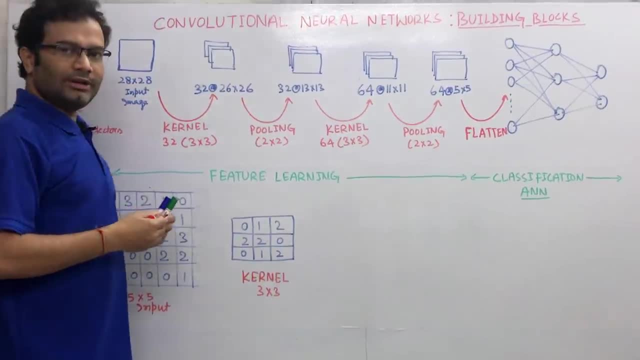 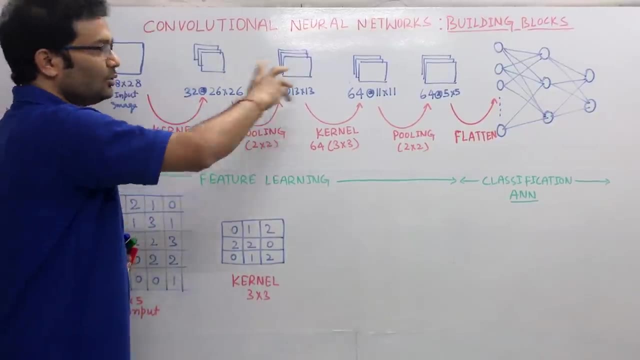 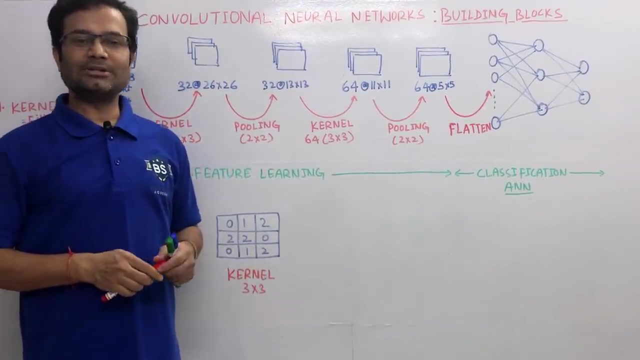 dimensionality. So suppose nowadays size of image very used 2000 by 2000 pixels or 4000 by 4000 pixels. So if you put direct those image in your classification or the fully connected network it would be the very expensive computation and it will take the time also. So where we use the 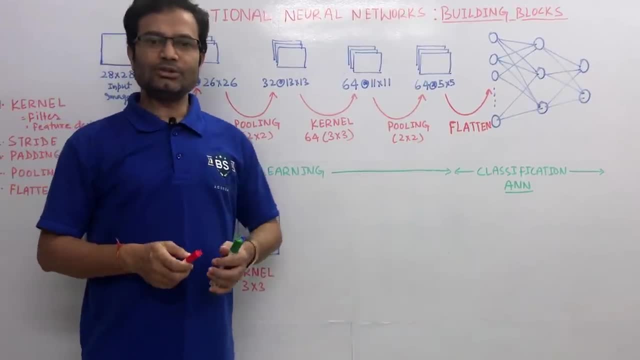 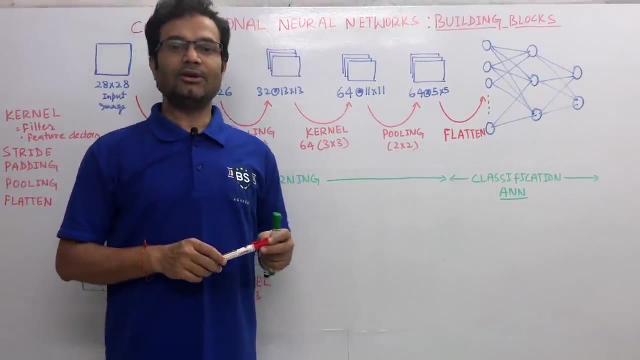 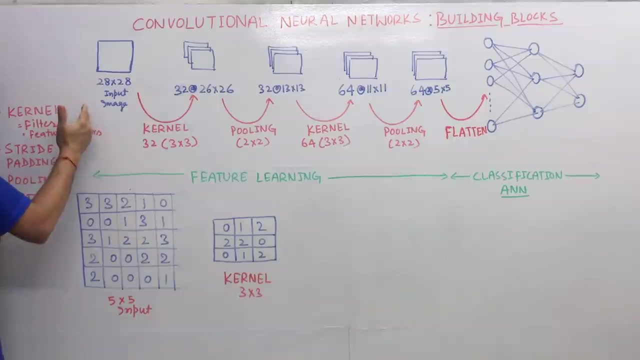 advantage of the CNN that reduce the image dimensionality in such a way to keeping all the important features for their good predictions, that help for the good predictions. That's why you can see here from here to here, this part is called the feature learning. So 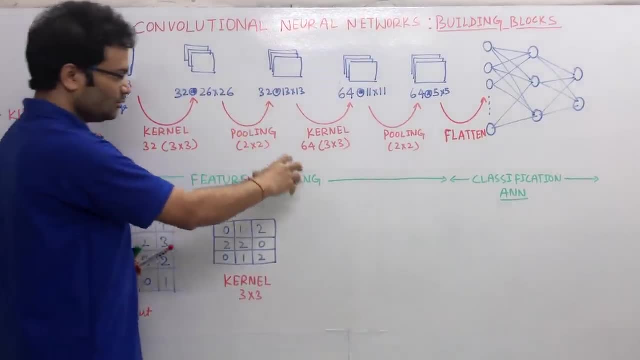 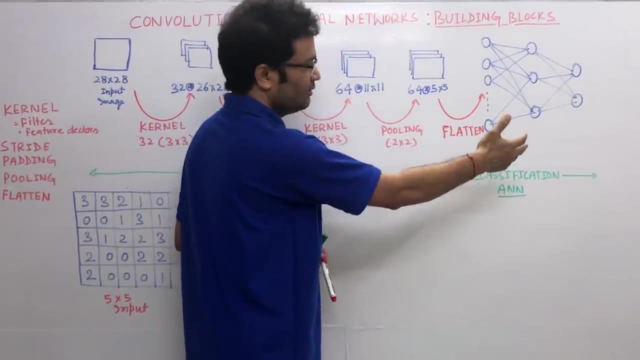 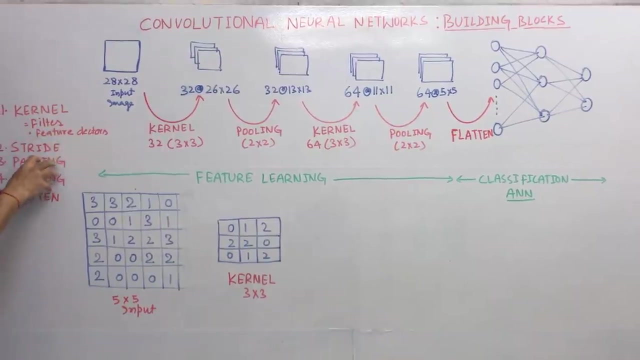 we are extracting all the important features. Once you extract, then put those data into the additional deep learning or the artificial neural network for their classification. So let us start. what is the important of each building block? So, first and important, I am going to use the 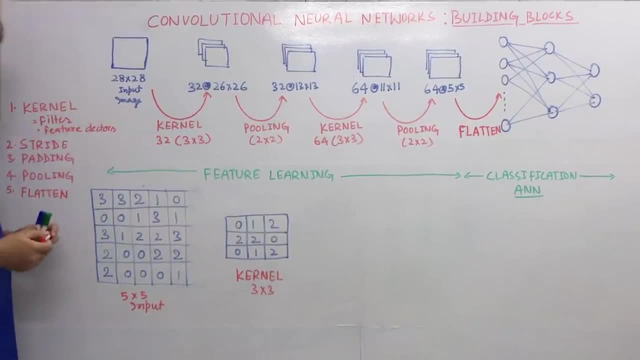 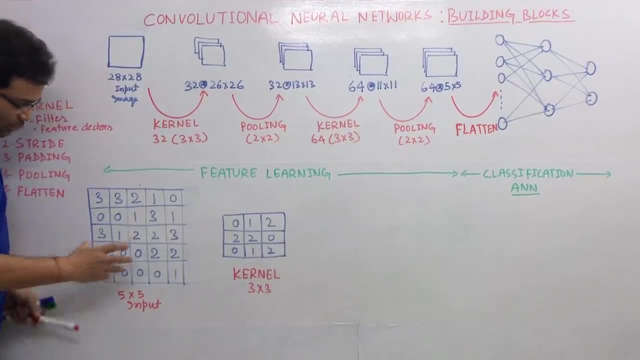 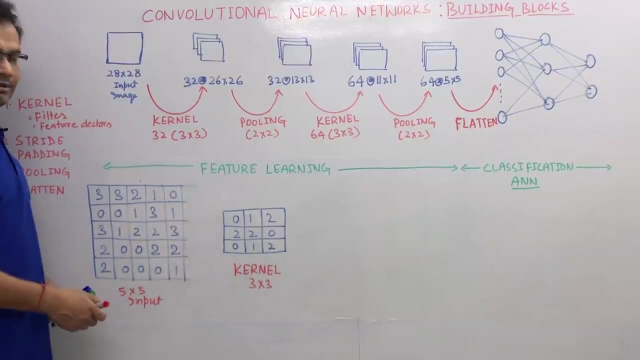 kernel, or we also call the filter or the filter detector. What is the meaning of that? So suppose you have the image 5 by 5, I have taken the small size So it will easy for me to explain all the mathematics behind it. So you see, 5 by 5 image is there and 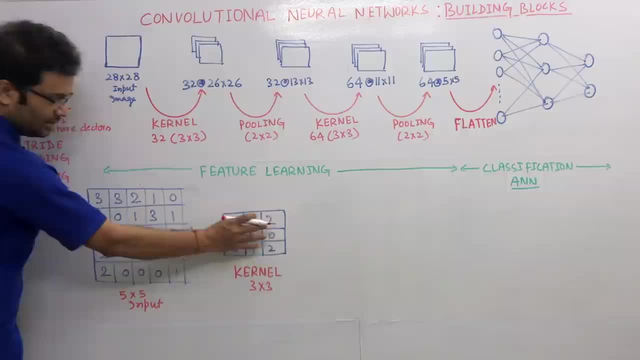 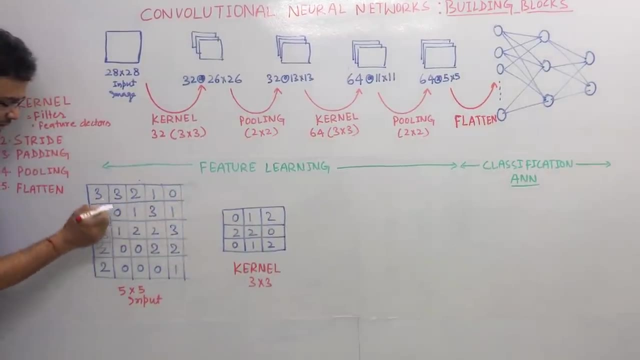 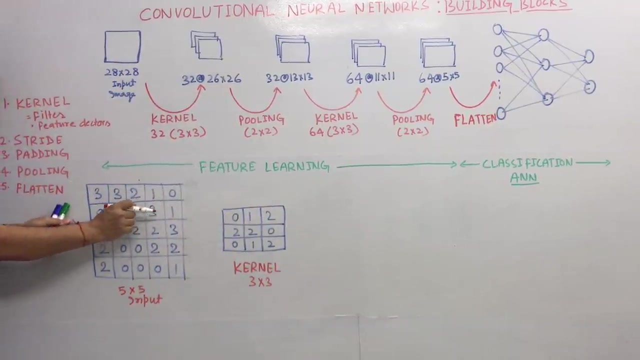 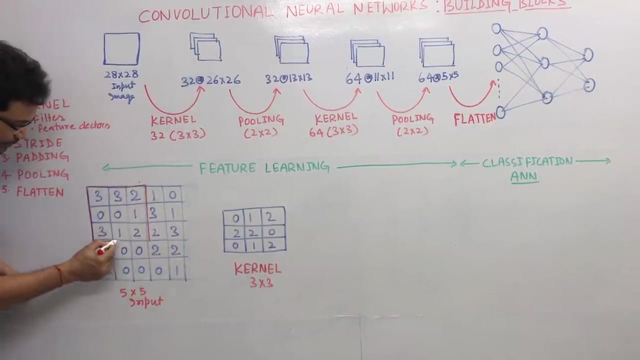 5 by 5 is the kernel What is called the convolutional. We will keep this image 3 by 3,. keep this filter on this image input 3 by 3.. So if you take this and keep it here from the left top corner, what where it will come? It will come here. Now. the image value is the 3,. 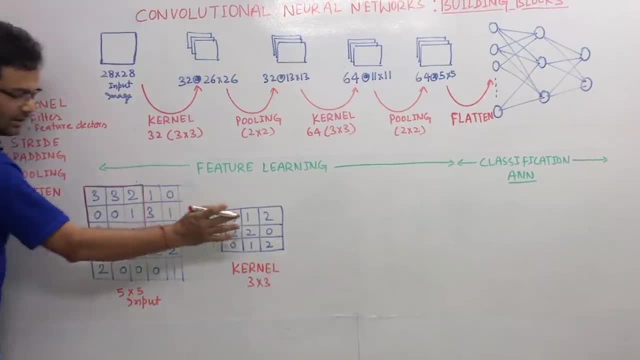 3, 2, 0, 0, 1,, 3,, 1, 2 and the kernel filter value is 0, 1,, 2,, 2, 2, 0, 0, 1, 2.. So 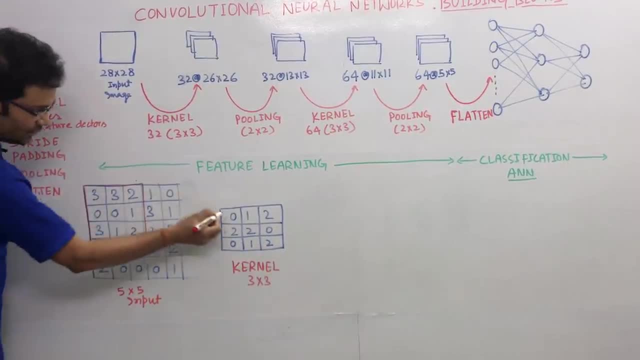 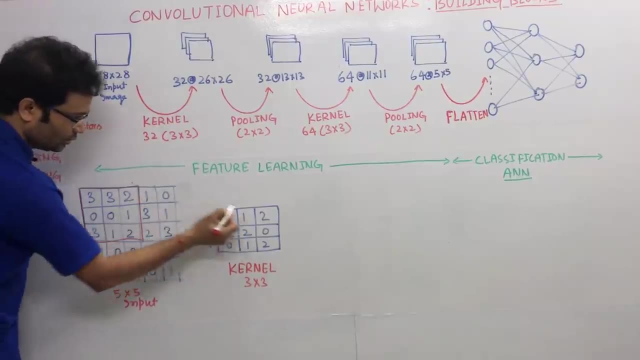 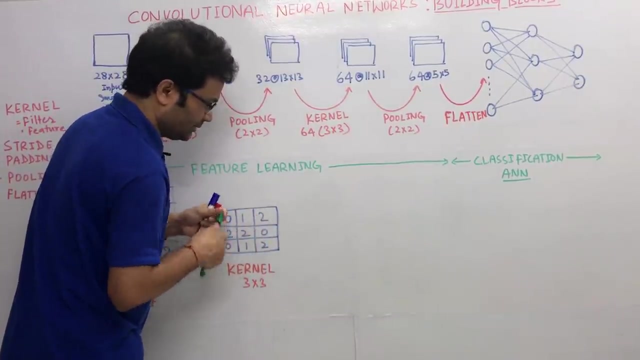 what will happen now? You have to multiply 3 into 0. So if you see here 3 into 0,, 3 into 1,, 2 into 2, the same way this 3 and this 3.. So let me put it here for the easy. 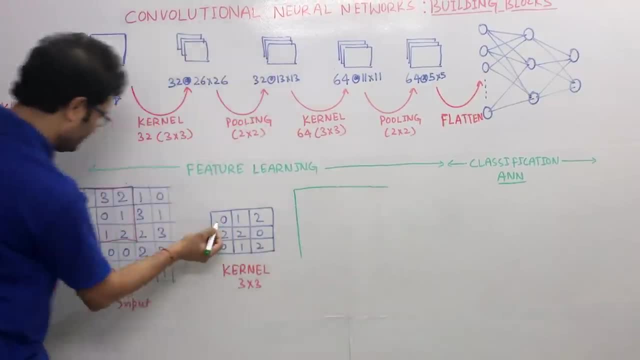 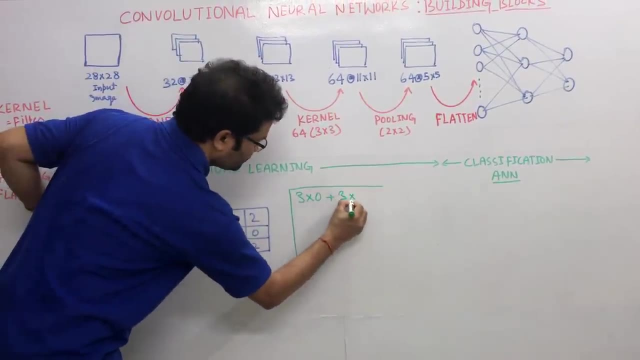 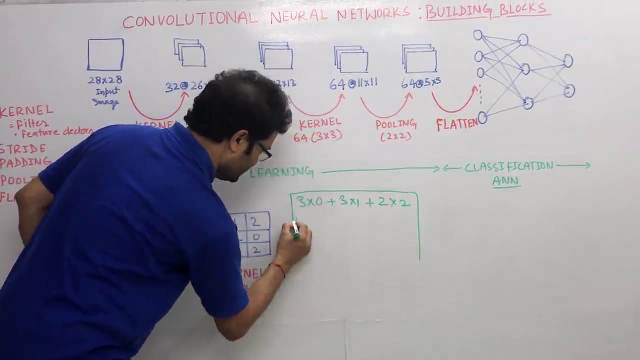 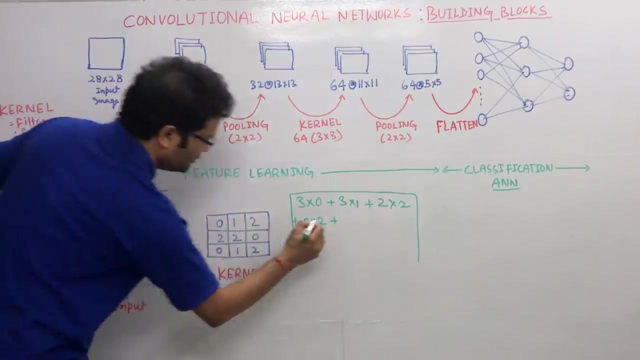 visualization. So what happened? This 3 into 0, you have to sum up 3 into 1, then you have to sum up then 2 into 2.. Then again, plus this 0, this 2, 0 into 2 plus 0 into 2 plus. 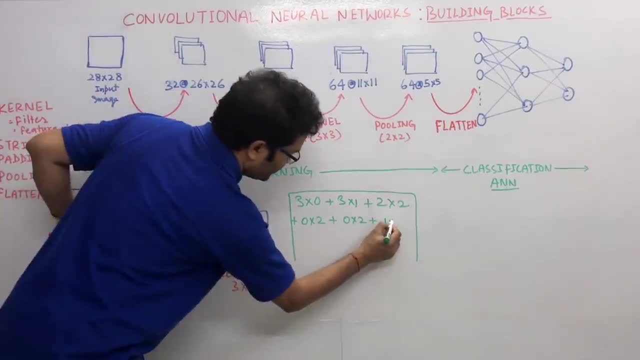 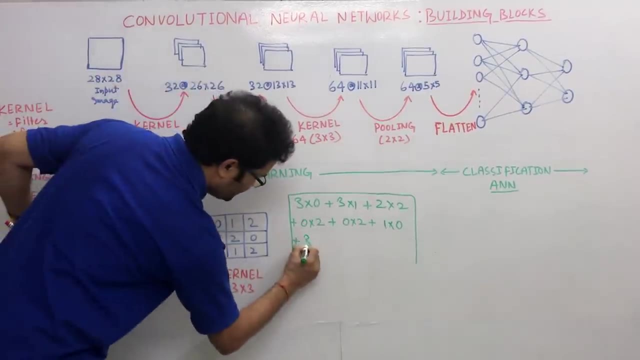 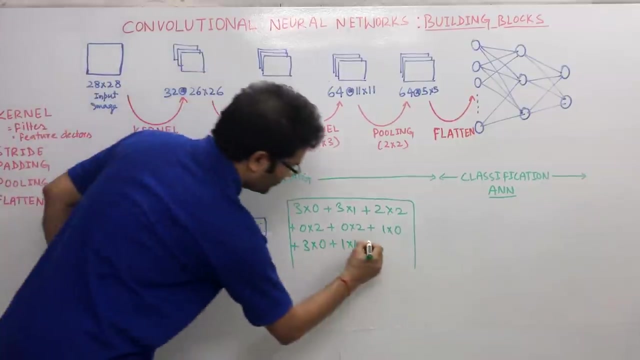 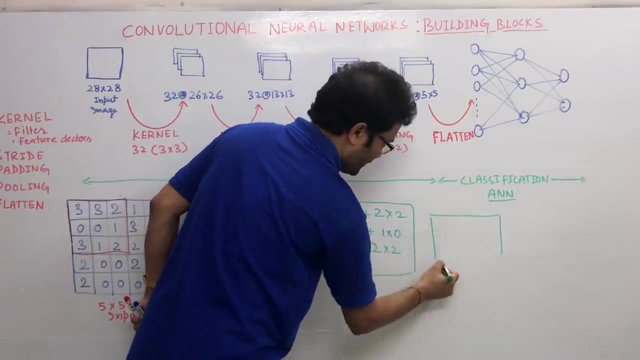 this 1 with this 0. So 1 into 0. Again, this 3 into this 3, 3 into 0, 1 into 1, 2 into 2 and then 2 into 2.. So if you calculate this part, what it become? 0 plus 3 plus 4. 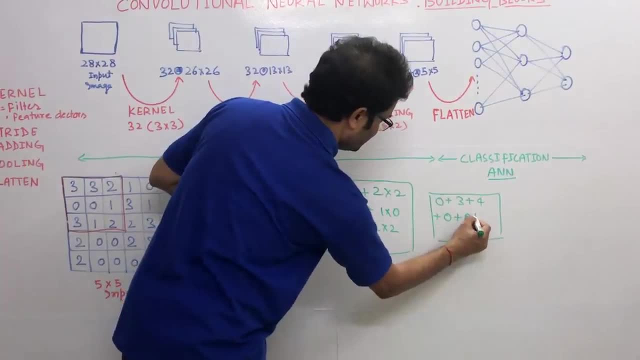 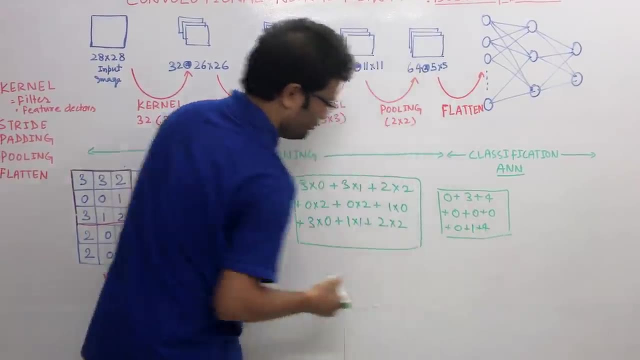 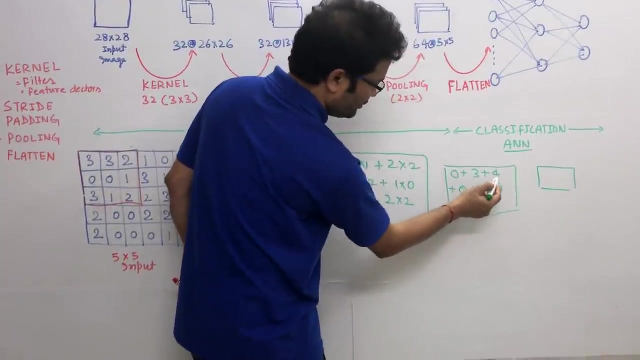 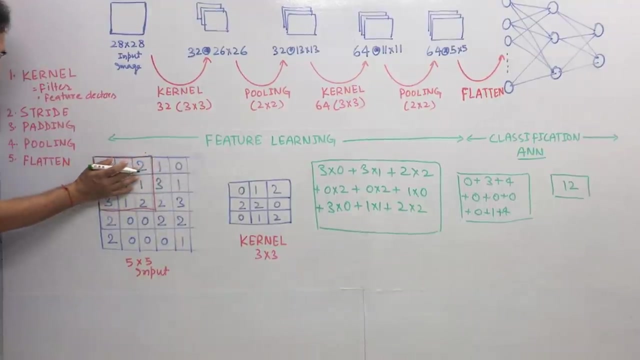 plus 0 plus 0 plus 0,, then again 0 plus 1 and plus 4, right? And then if you add at the end everything, it become the: how much? 3, 4,, 7,, 8,, 12, right? So output of this: 1 convolutional. 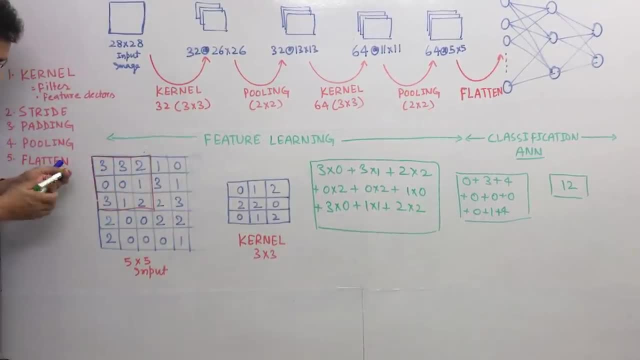 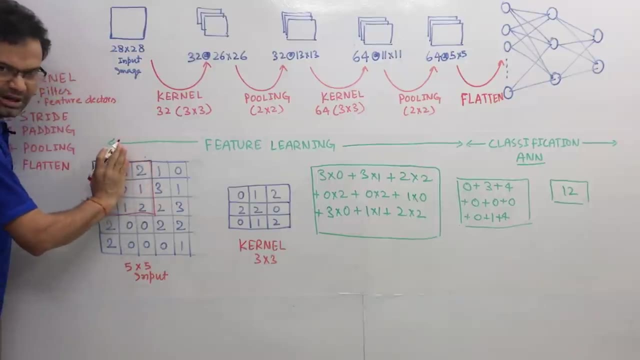 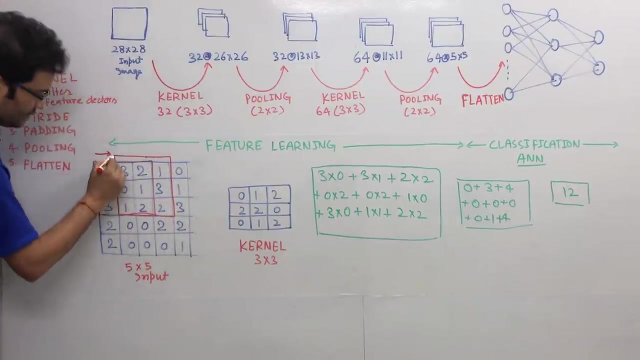 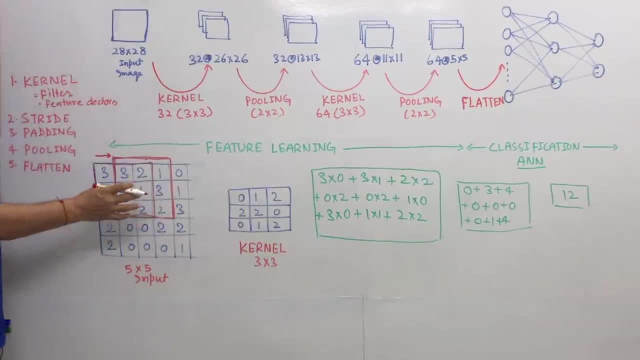 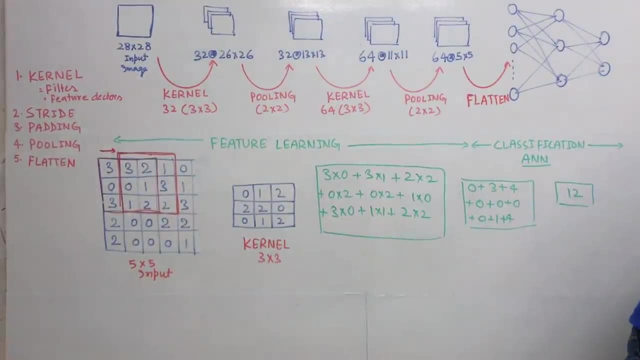 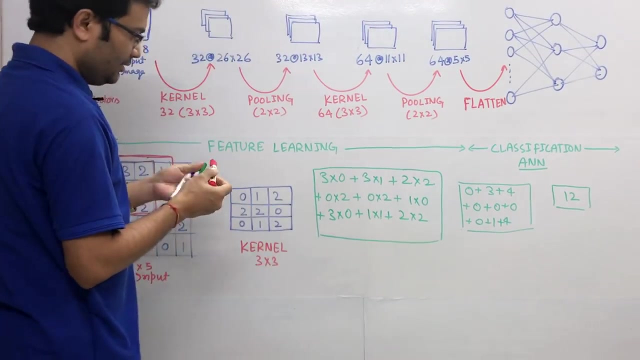 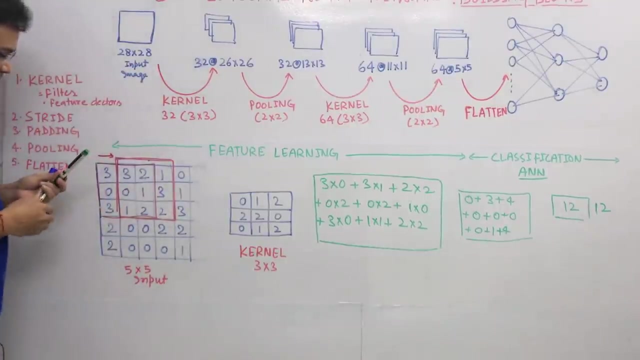 So it will come here right. Then again you have to calculate and you have to put the value. So again, if you do, the value would be the 12. And then again what you have to do Again after this, again you 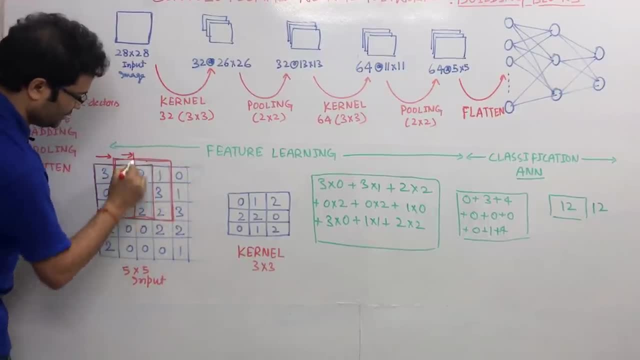 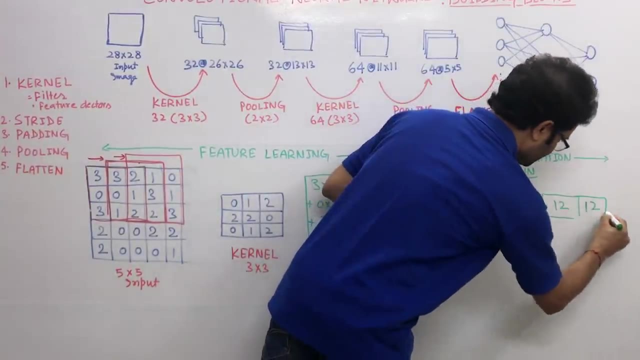 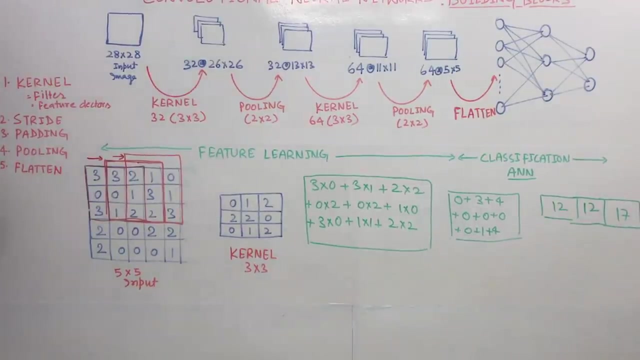 have to move right, one step by one step. So this is the third part, So it become the 17.. Now what you have to do Now. this upper part is done, So now we move to the right. 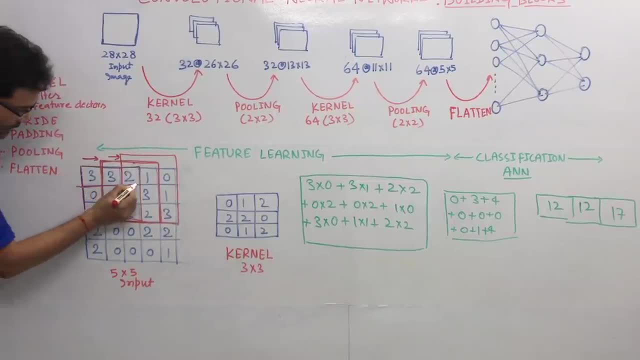 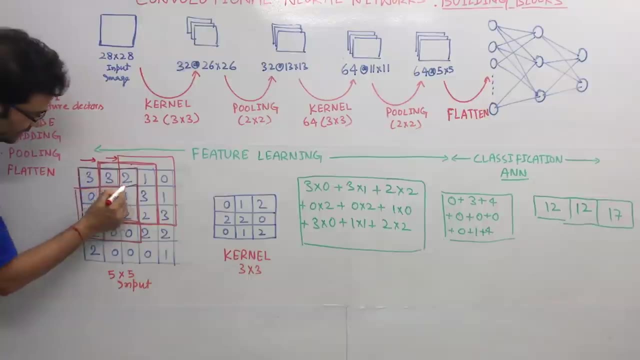 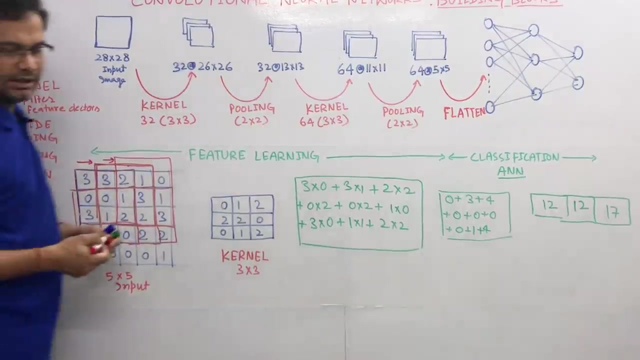 side. You have to move the now down. So this time this one right. Then after this we move to the right side. So now this one, then after this this part, after that this part. So again we have the 1,, 2,, 3 and that. 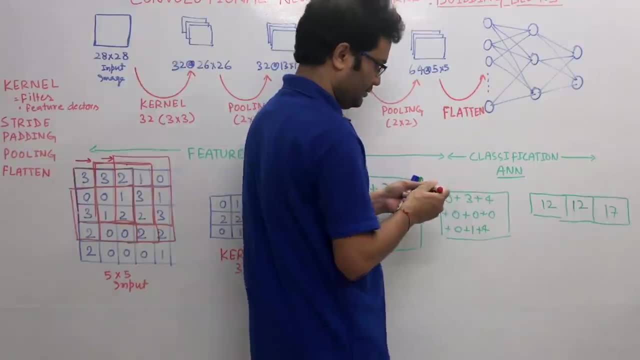 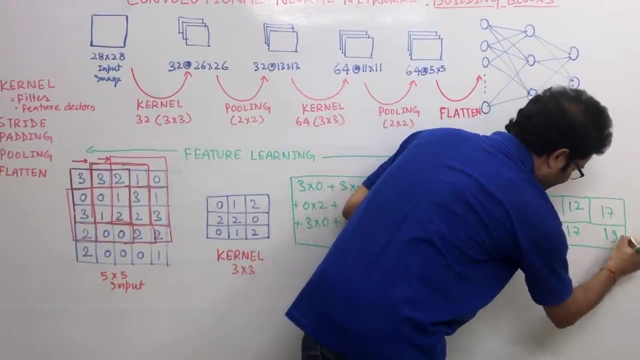 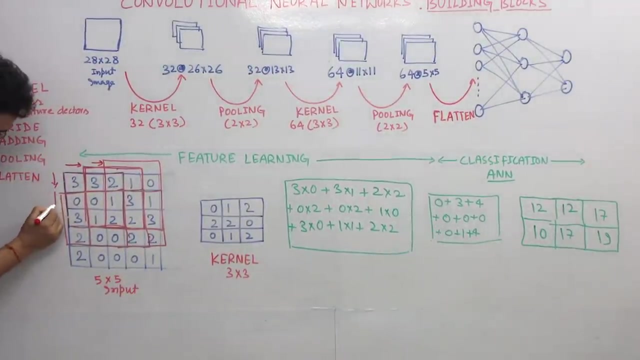 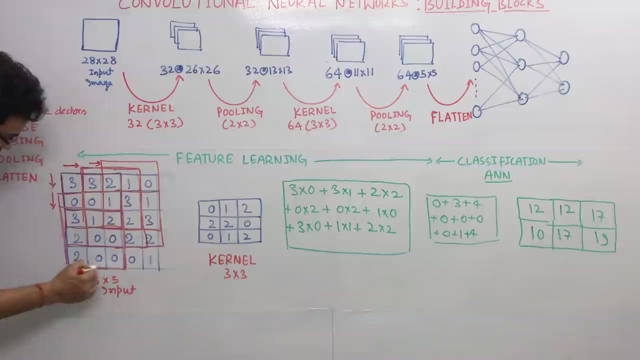 value is 10,, 17,, 19.. So this value is 10,, 17 and 19.. Again, we have to move one down right, So it become here right, this part. this let me put in different color, So it 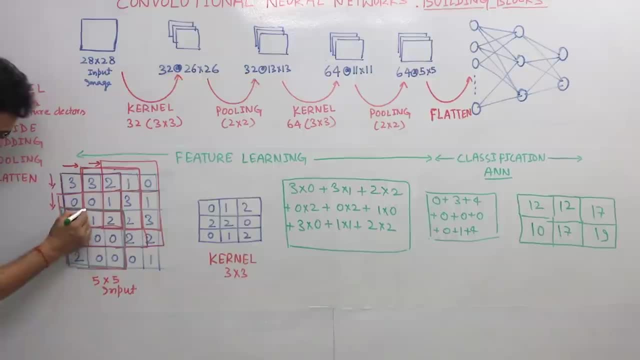 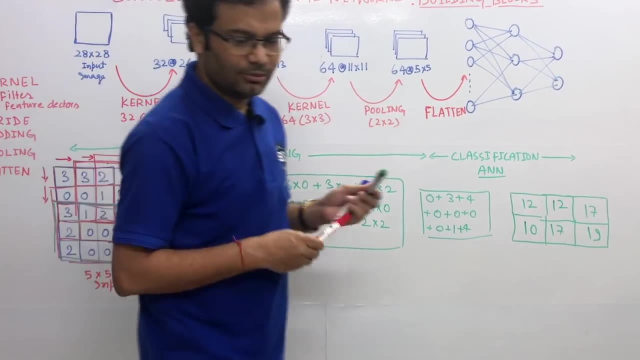 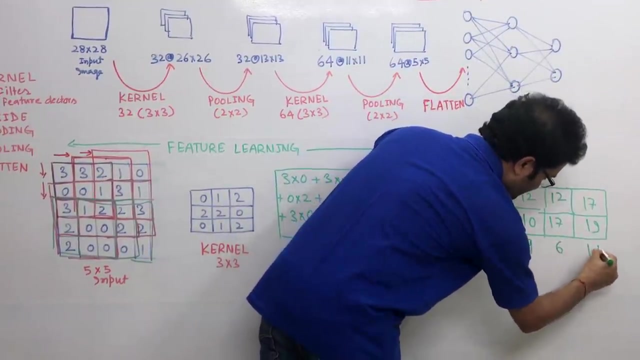 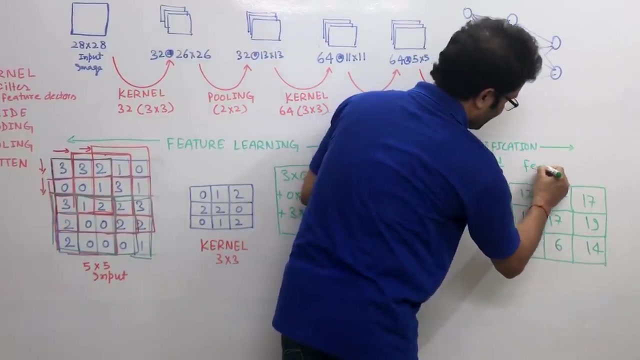 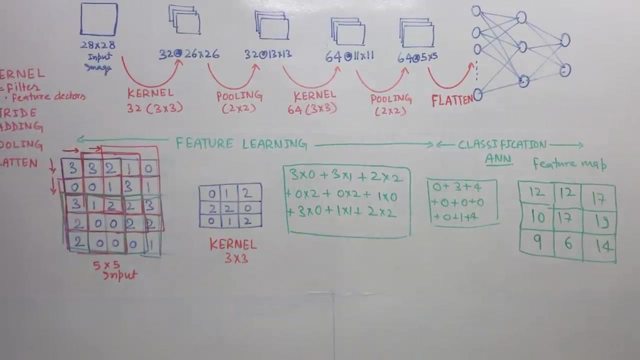 easy for you. this part 1, again towards right, again here. So again we have the 3 value right. that value become the 9, 6, 14, 9, 6, 14.. This is called the future map or the convoluted map. So now you can see that we have the. 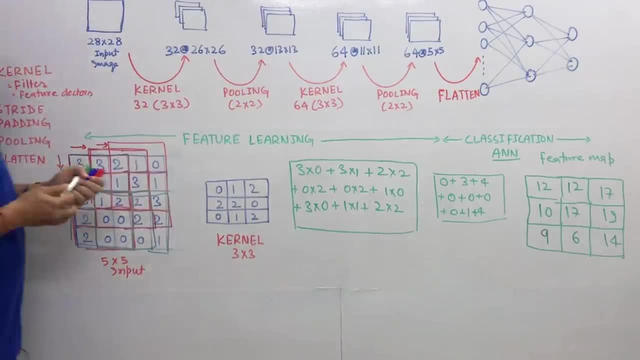 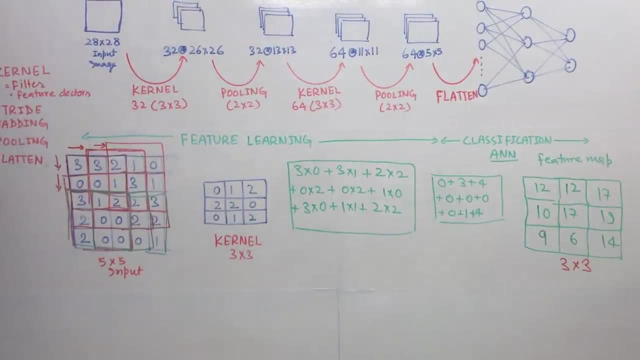 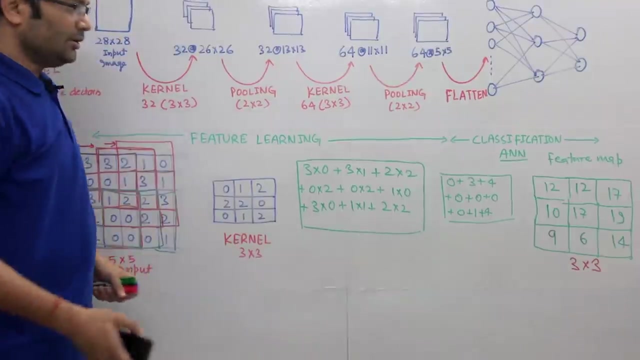 input 5 into 5, we use the kernel and it become the size of the 3 into 3.. So do you have any formula who can directly tell me what is the? what is the size of the kernel? So size of the future map. So I think we got one formula here. we can use this formula. 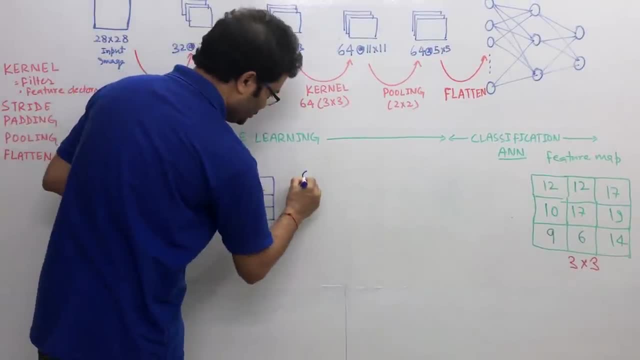 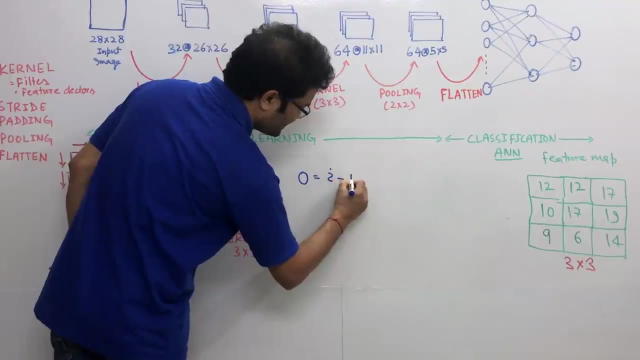 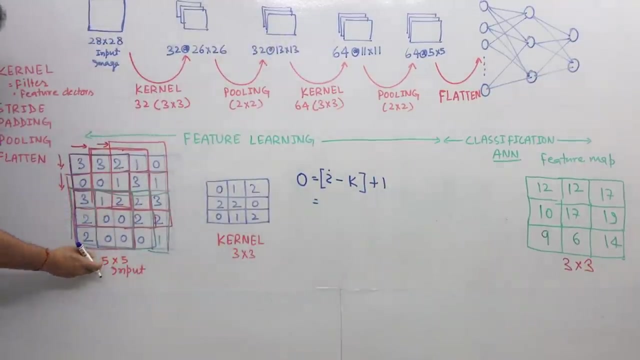 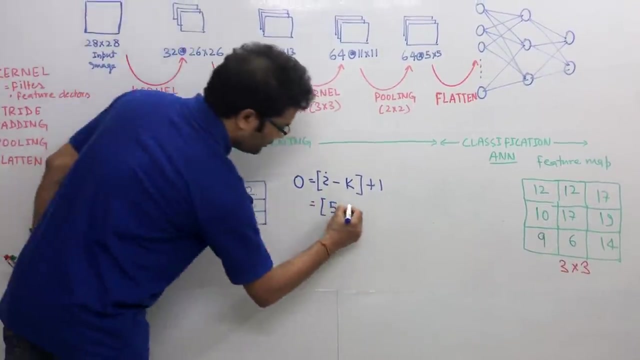 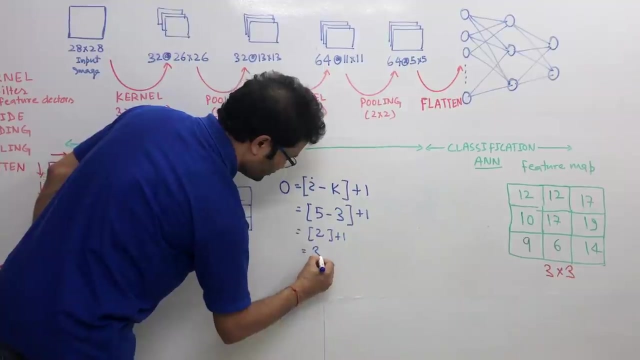 So what you have to do? output is equal to size of input minus size of kernel, plus 1, see if it work or not. So 5 by 5, take the 5 only, and size of kernel 3, take the 3 only and 1.. So 2 plus 1 is equal to 3.. So we got the 3 by 3.. So this: 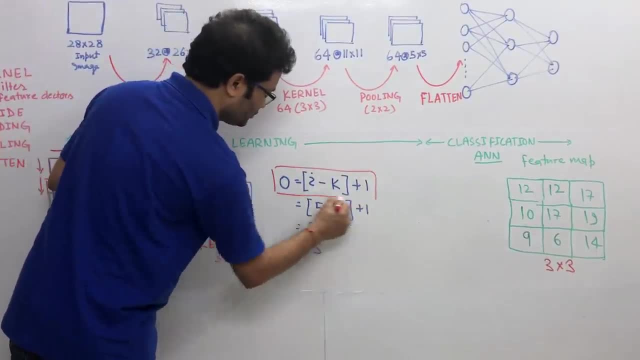 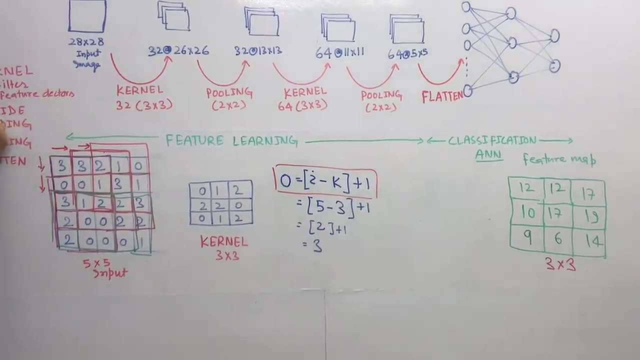 formula. we work if you use only the kernel concept, right. So now I am going to use the stride. What is the stride? Stride says not only the kernel concept, but also the kernel concept. So what is the? 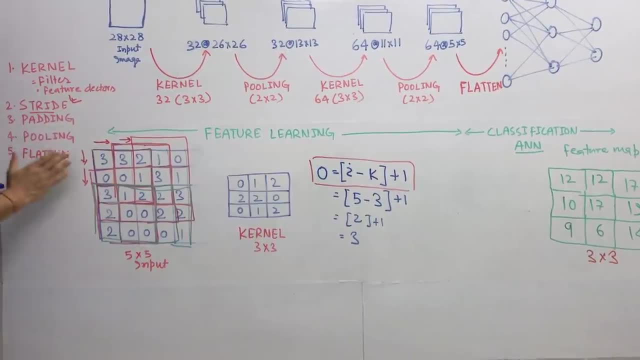 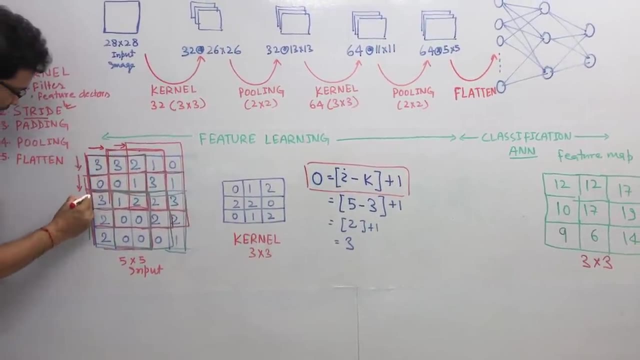 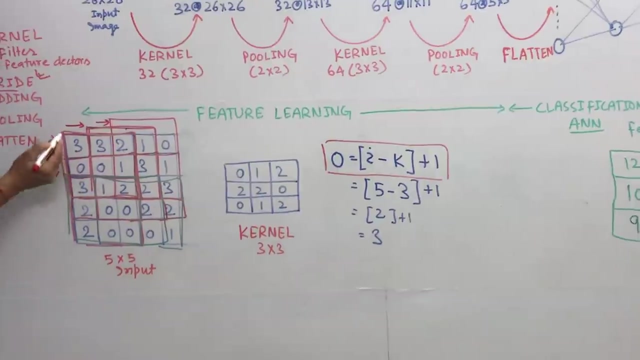 stride. Now if you see, we move one by one right. So what happen if you see, take the first again, it was the first right, take the first After that from where we had started just 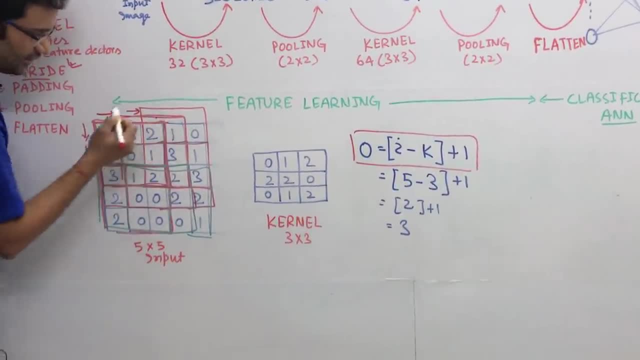 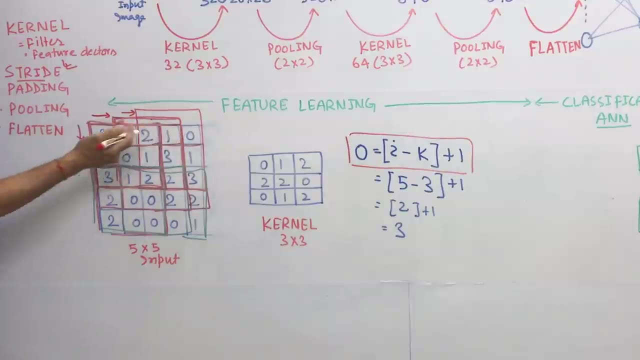 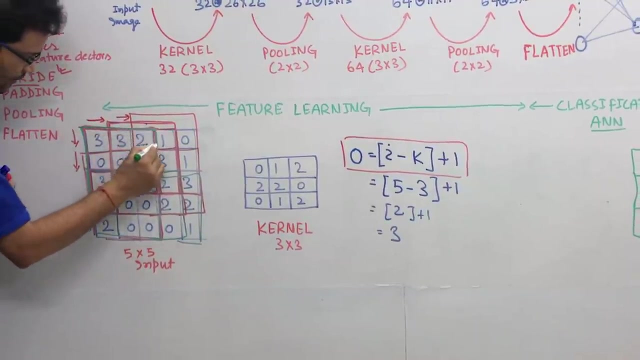 one box there, right here. right, it was here, right, So instead of the 1, you move the 2 block, So I will not start from n. So if this is, if it was the first 1,, this the first 1, second will not start from. 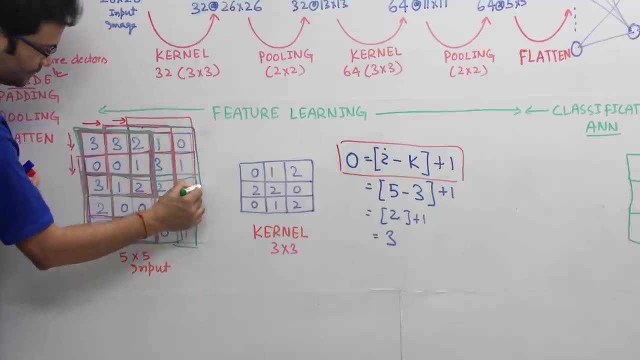 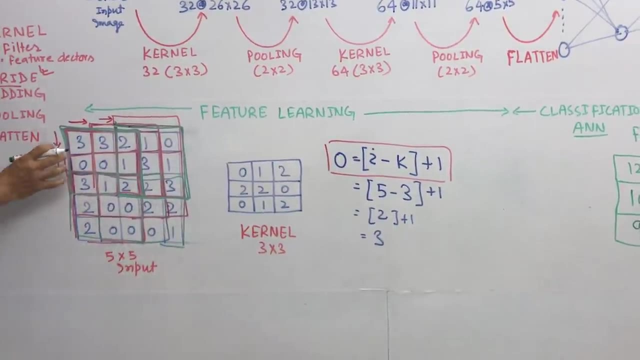 here. second will start from here, And you can see that I am done. means even for the true move. I capture all the values. So 1 and 1, right. So output would be set to n If this is the first one. 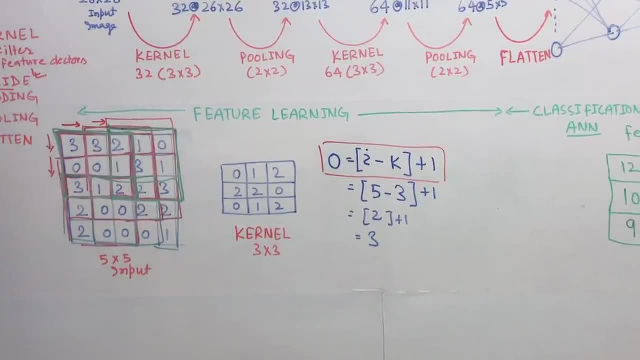 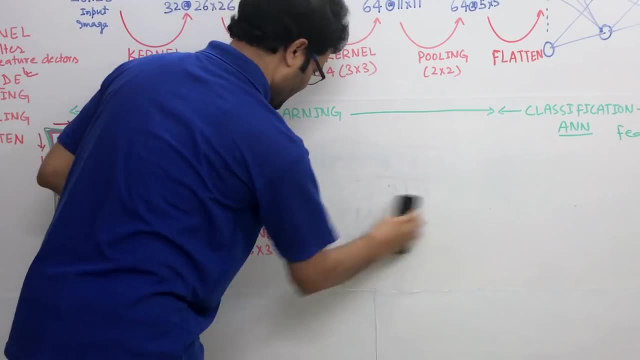 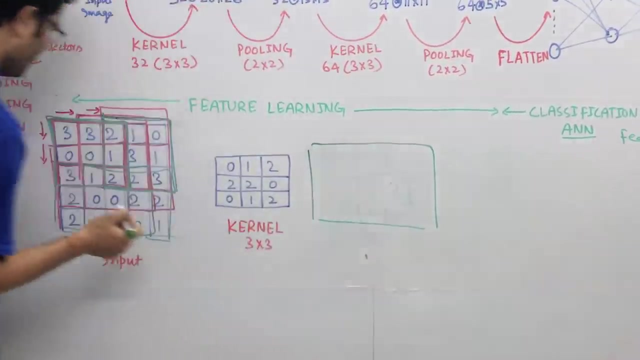 Only that this is a node, that is node itself is a node And it is taken from here. It is taken. this company benefit here. output would be the not in this formula. So now output will happen, see. take it here first. 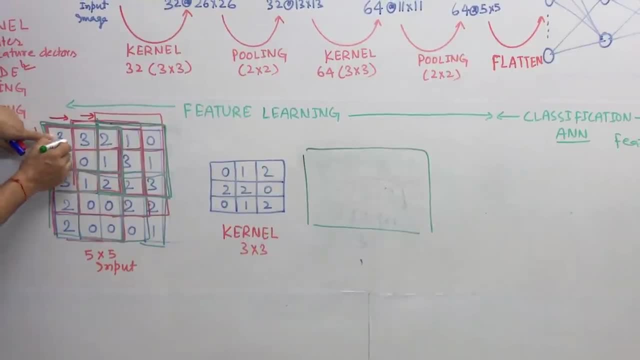 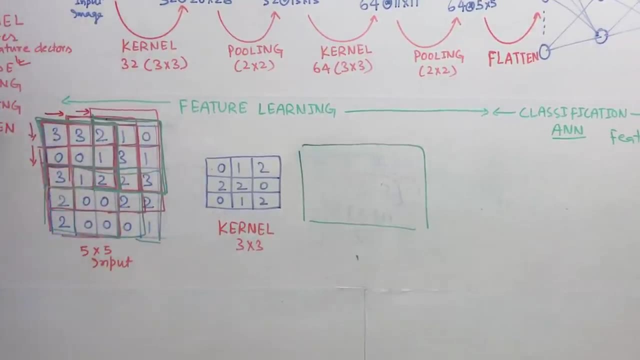 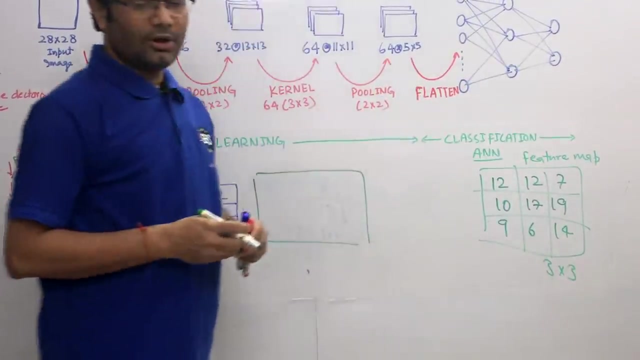 is the same output, how we calculating 3 into 0,, 3 into 1,, 2 into 1, then the 3, 2, 1. here, right and second case, we can directly move into that part. So earlier if you see, 3 into 3, now if you see we are not considering middle one. So 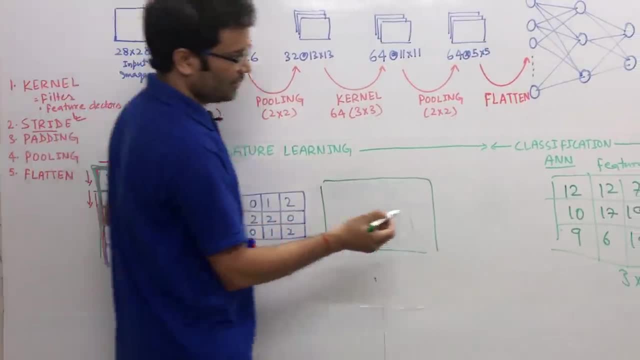 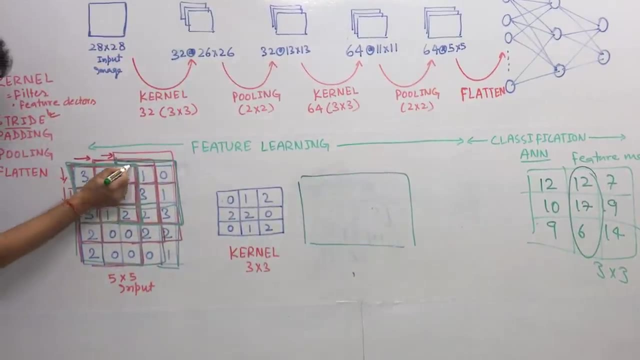 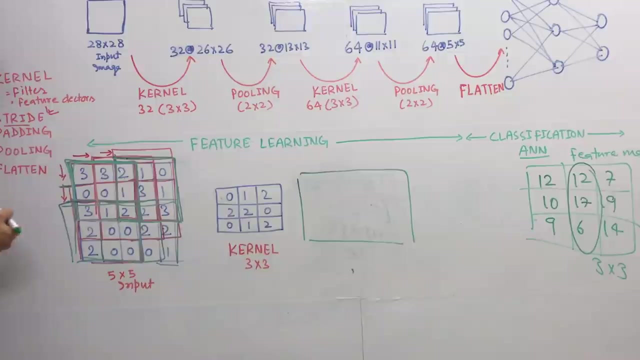 from here. I am going to last one. So in this way I am not considering this part, right? The same way, if you take the down from here, I will not start from here. I will start from here, right? So if you see one by one, this, we also divided. 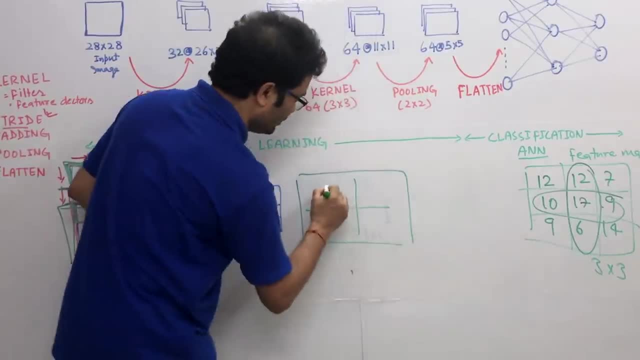 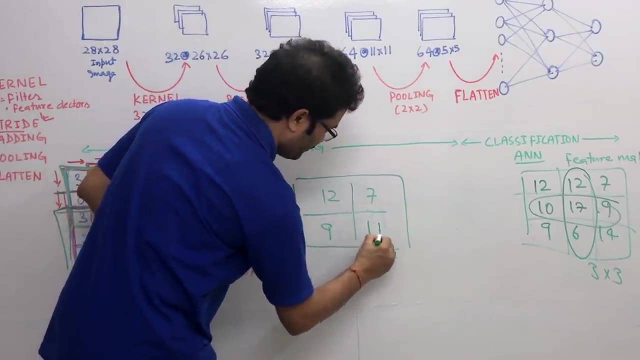 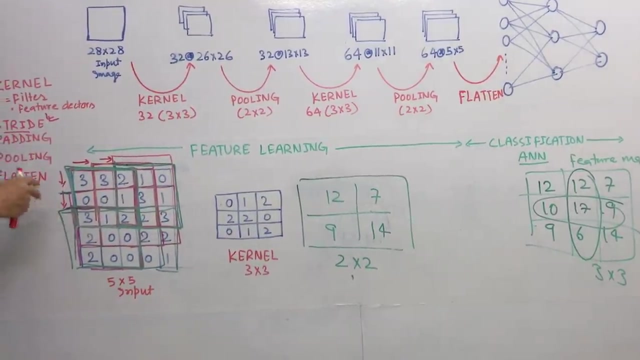 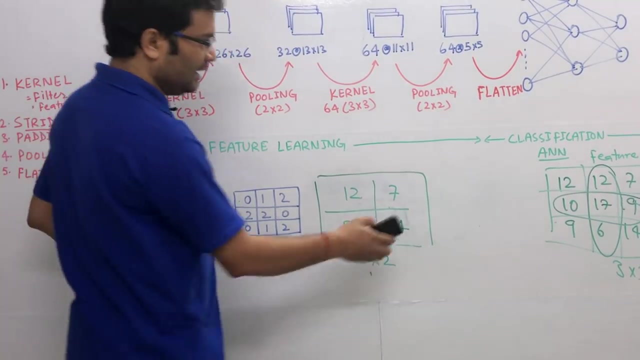 So only output will be there: 12,, 7, and then 9,, 14,. it become the 2 by 2.. If you use the stride 2, my dimension become the 2 by 2, right? So can we derive any formula here? I think? 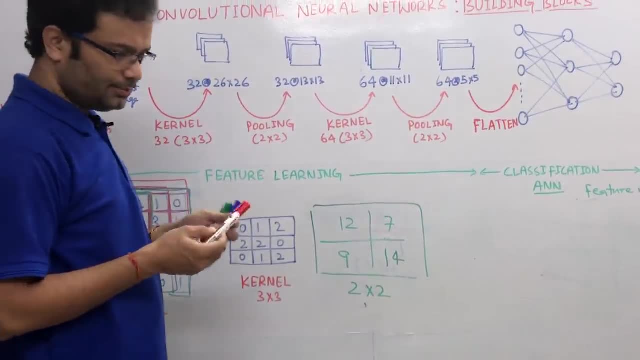 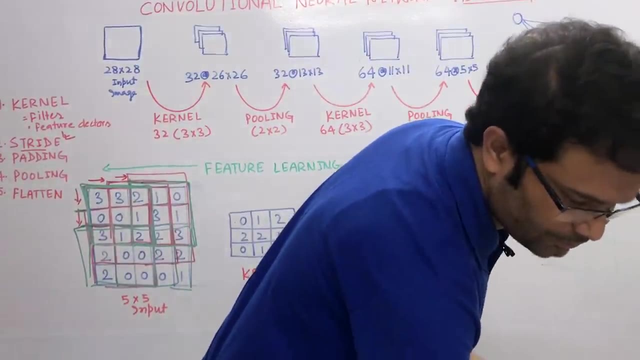 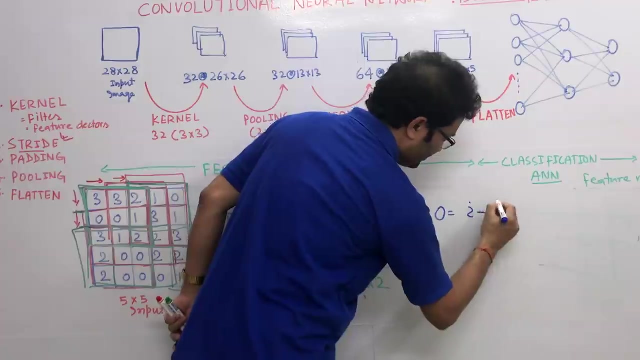 yes, we can derive the formula: What we have to do, So what we have to do, So what we have to do, So what we have to do. We can use the, we can use the. output is equal to the same formula: I minus k divided. 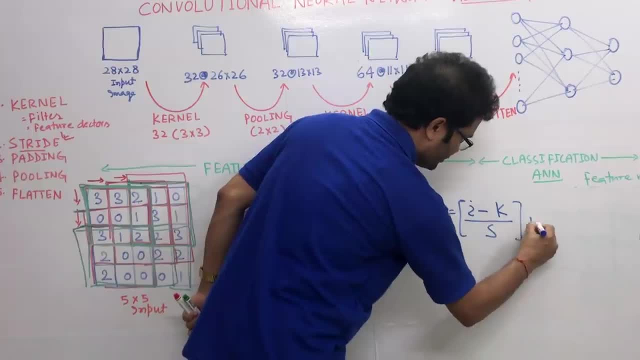 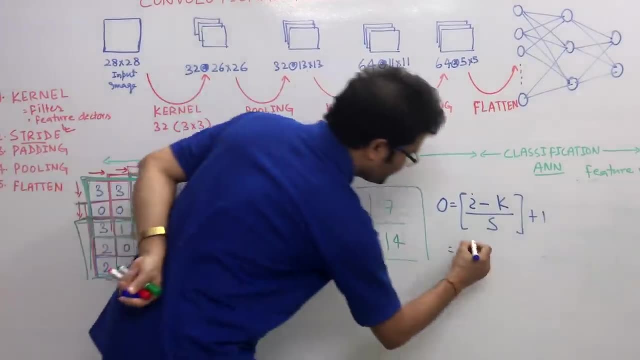 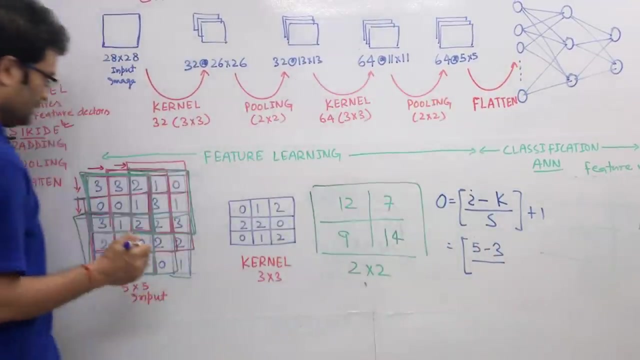 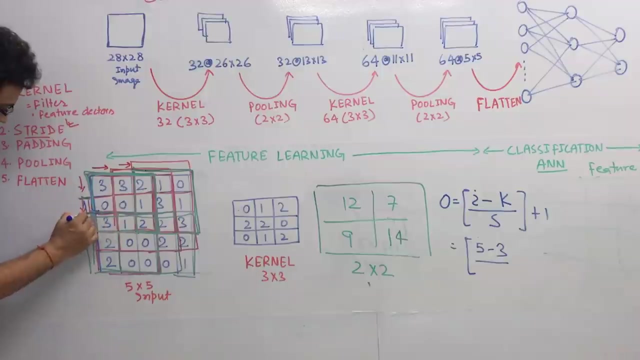 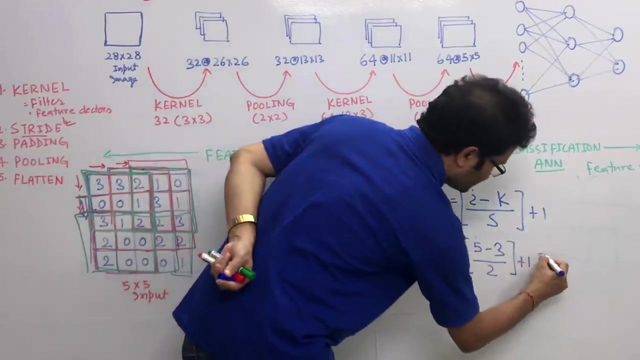 by stripe n plus 1.. So how it will work, I was the 5. here minus corner is the 3, stripe. I am moving 2 stripe. ok, So it was here directly, coming here, right? So this 2 block I am moving at a time. So this is the 2 and plus 1.. So 2: 2 answer is 2. So 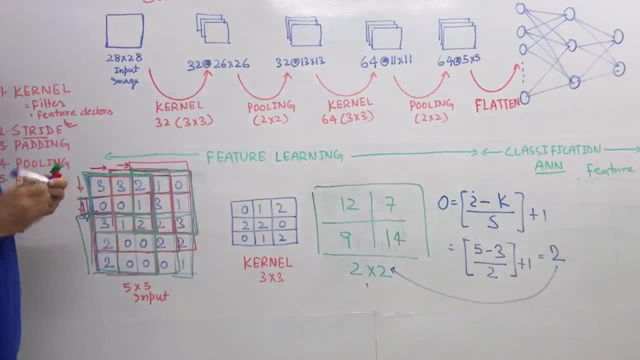 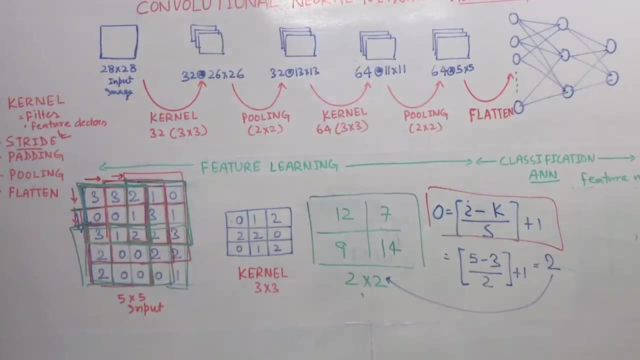 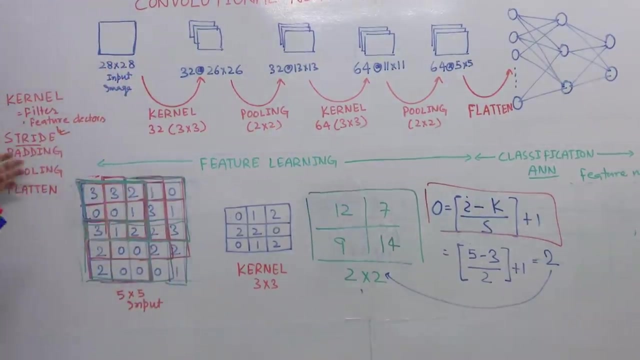 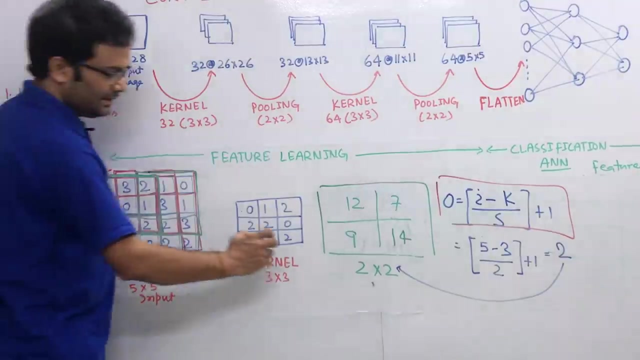 you can see that we have the 2- 2.. So this is the formula. if you have the any stripe in your input block right Now. the third concept is: come the padding. So padding, padding is says. So now you see, we have the input 5 into 5, but getting the output either. 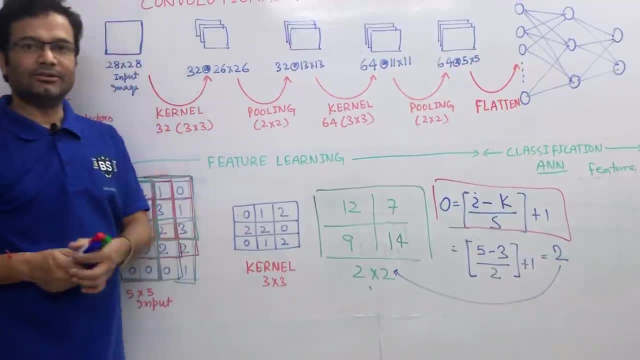 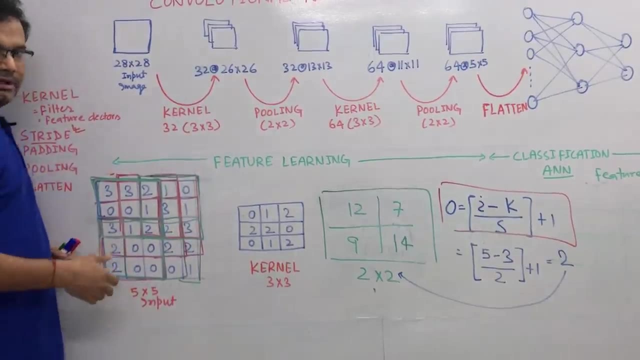 2 by 2 or in the previous example it was the 3 by 3.. So somehow I am going to lose some information that was in the form of 5 by 5. that is not possible in the 3 by 3.. 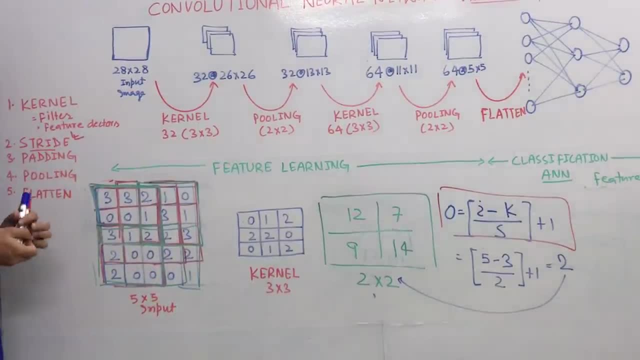 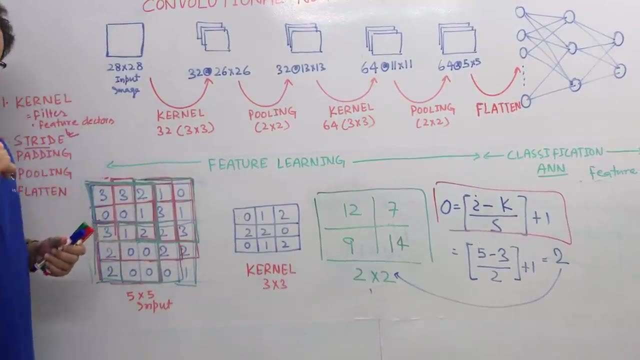 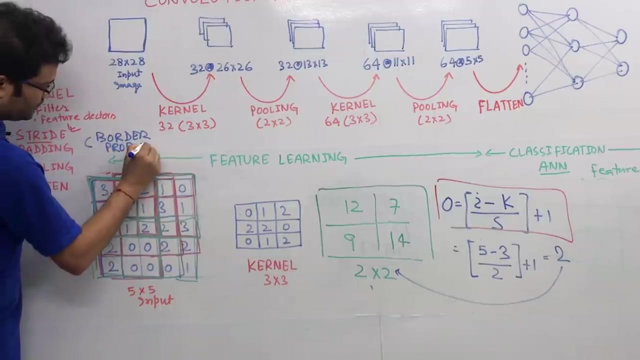 So padding is saying that I have to preserve the same information. how we can preserve this is the one thing. And second thing for the padding, if you see that is padding is also called the border problem. Why border problem solver? Why it is called, If you see this: 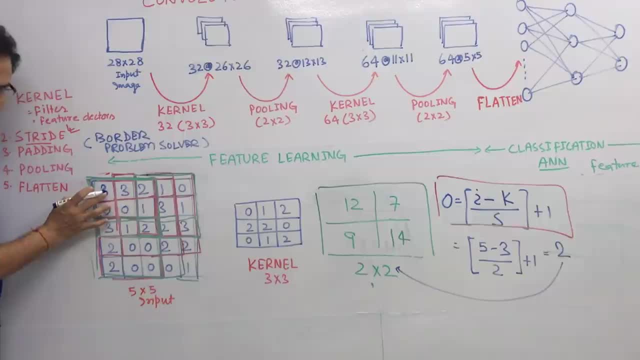 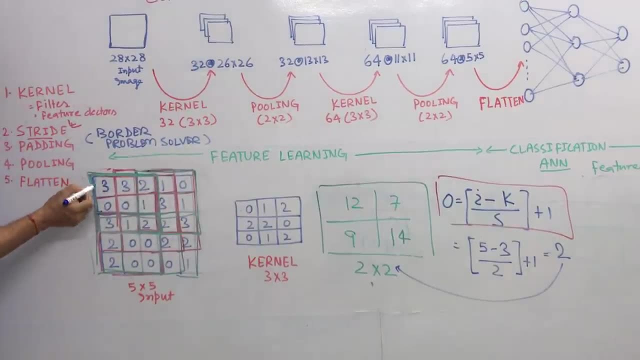 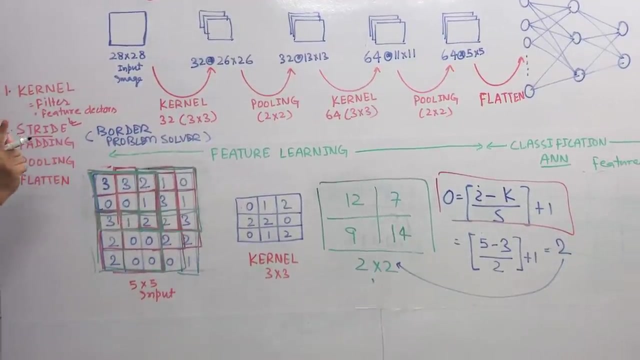 the input image. these three. that is on the border. they are not getting the chance to when the filter move over here. So this is only one time it get the chance right. When I keep this filter over here it got only one time chance, But if you see these three, it got the two time chance. 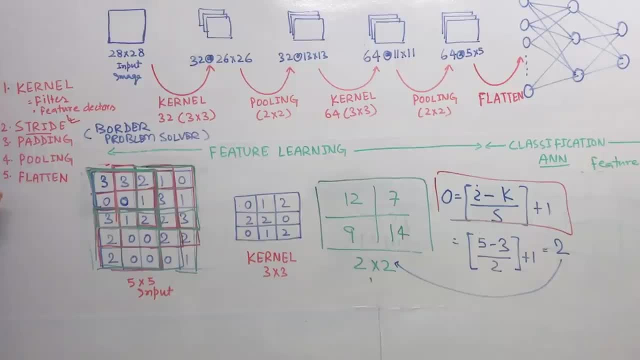 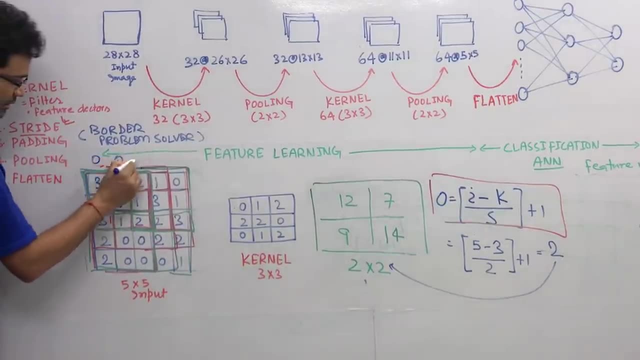 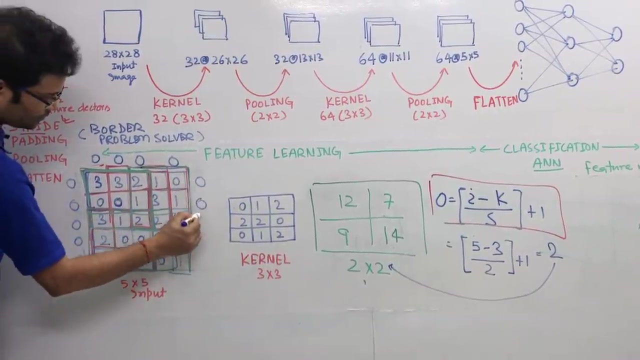 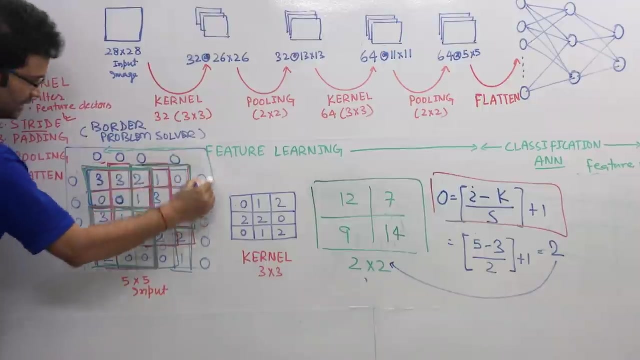 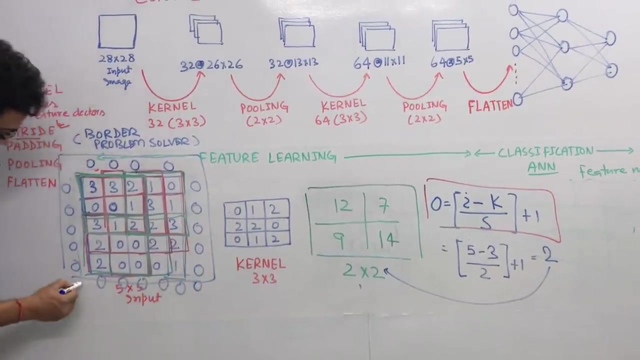 If you see this part, this got the three time chance. So to solve this problem, what we will do is we put the one zero padding all over the input. So now, if you do this diagram- see bottom here also- So we are adding the zero padding. 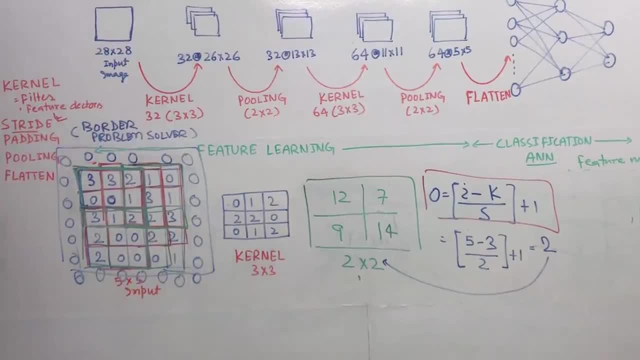 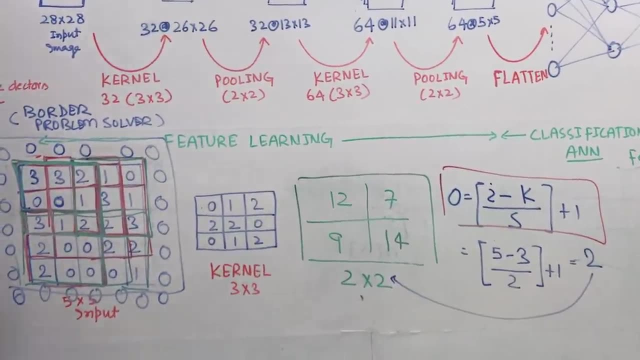 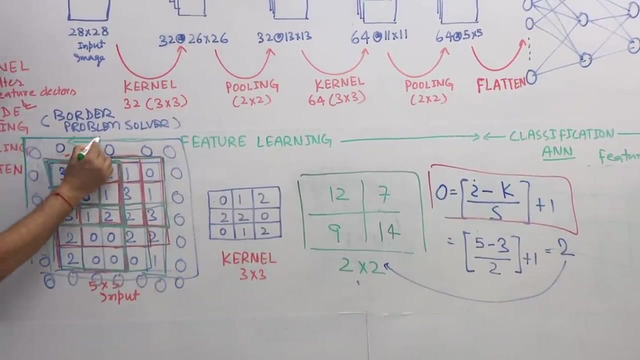 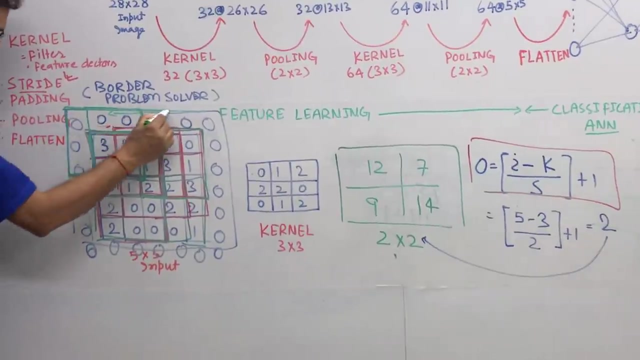 over all the four side of the input image, Then if this is the input, then if this is the kernel, what is the output? Then if you see, now, if you move this kernel, this kernel, we move here first move and then the second move, So I am direct writing the first kernel. 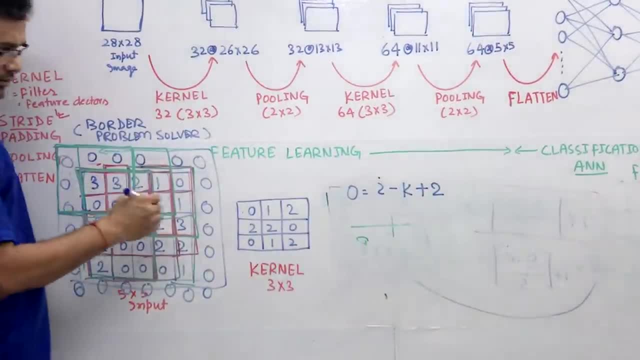 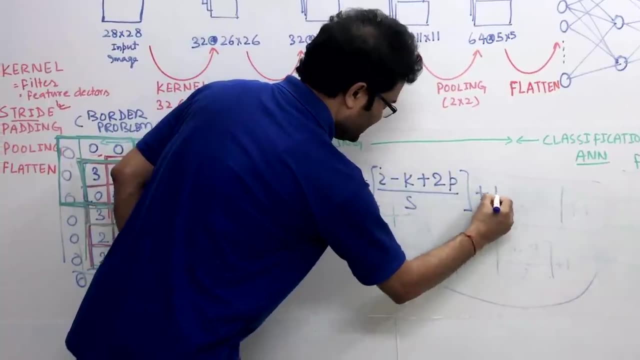 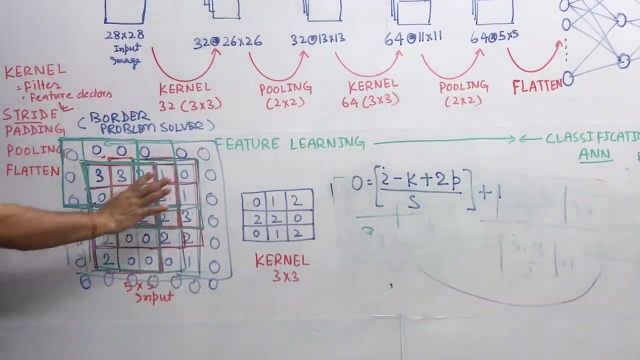 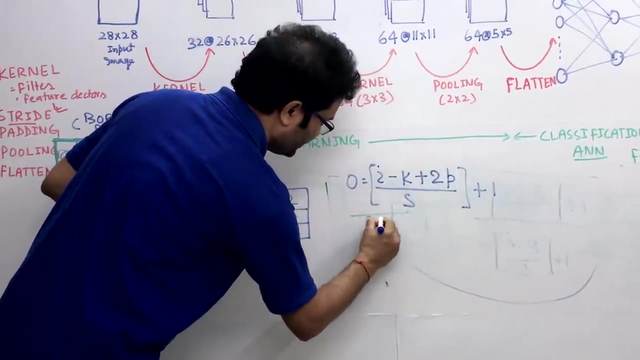 First two into this padding: P divided by S. This is the complete formula. So in this case, what will happen? I am not going to the stride. So this s is equal to 1 and the I is equal to. as usual, we have the 5, kernel is equal to 3.. I- 5,. 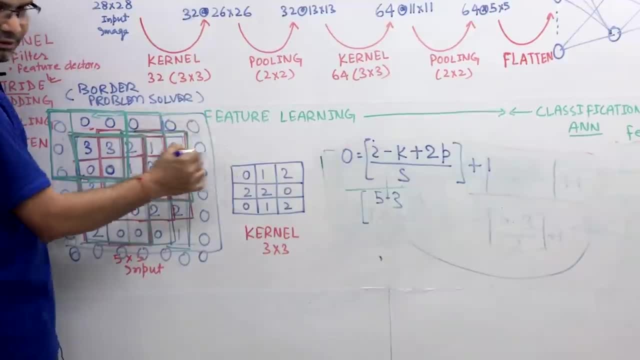 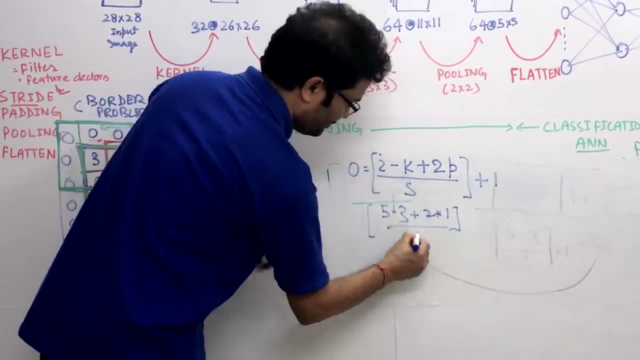 kernel 3. And we have the singlet that is being set. So if I select cut, then basically this is a and we have taken 1 right, or the 4 side is 1. 1 move So 2 into 1. we do not have any. 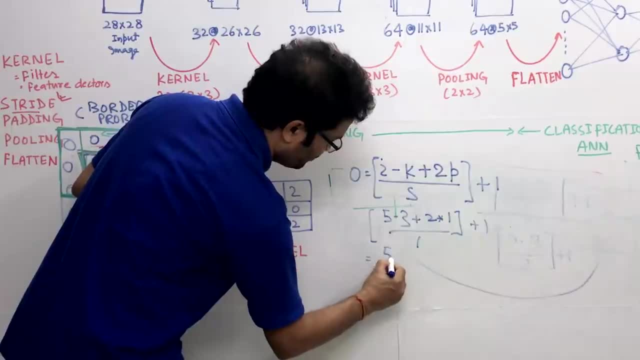 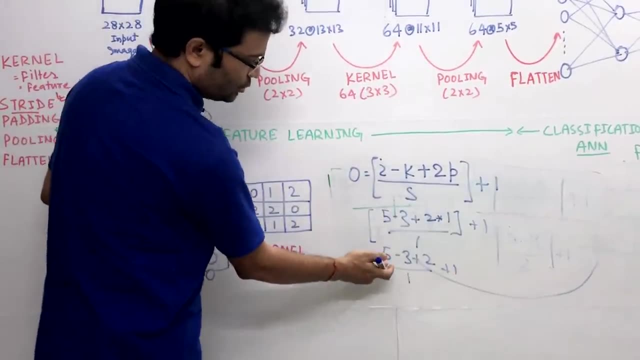 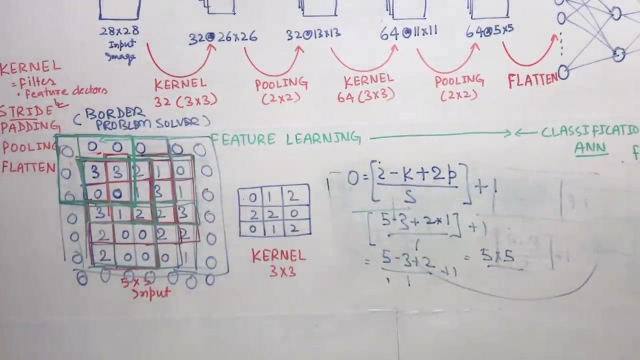 stripe 1 and plus 1.. So if you do 5 minus 3 plus 2 by 1, nothing and the plus 1.. So 5 minus 2, 2, 2 to 4, it become the 5 into 5.. So now you can get the question, or you. 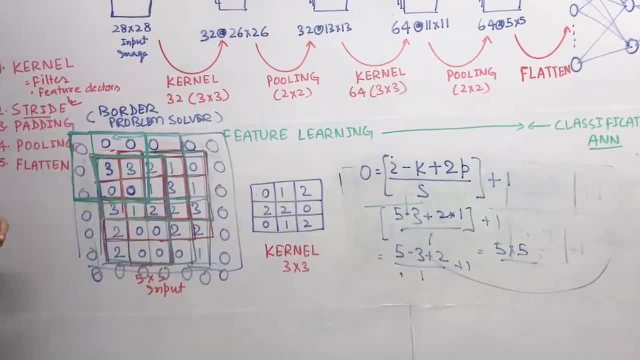 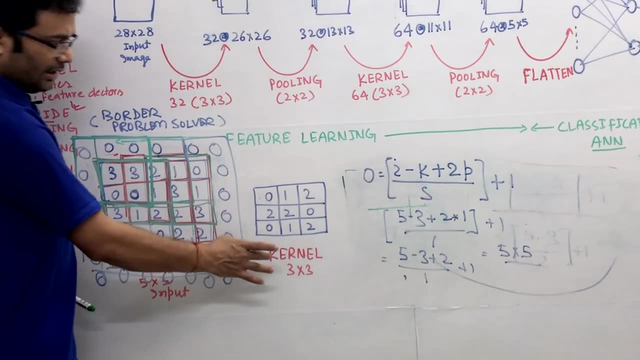 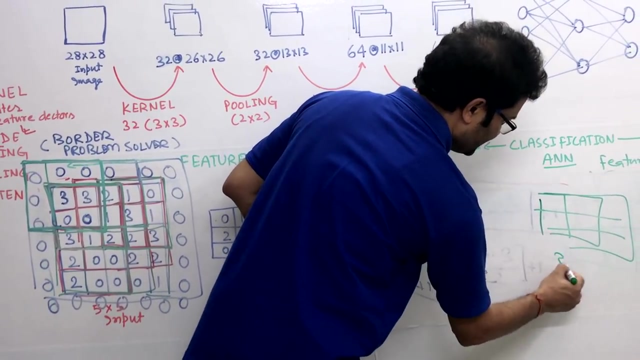 can. you can, you can implement in this way or you can. I will show in the coding. So if you use the, you record the first one- it was a 5 by 5- and use the kind of 3 by 3. our output was that the 3 by 3 right To preserve the same information. if you want to make the 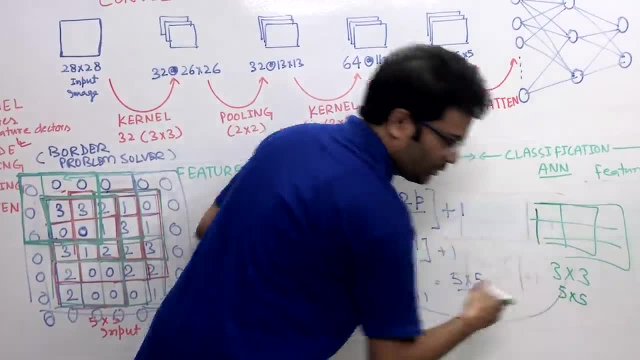 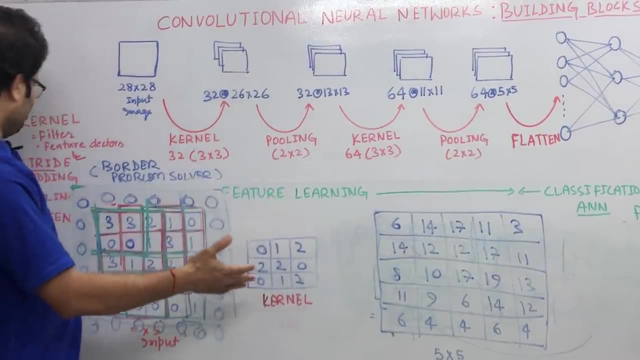 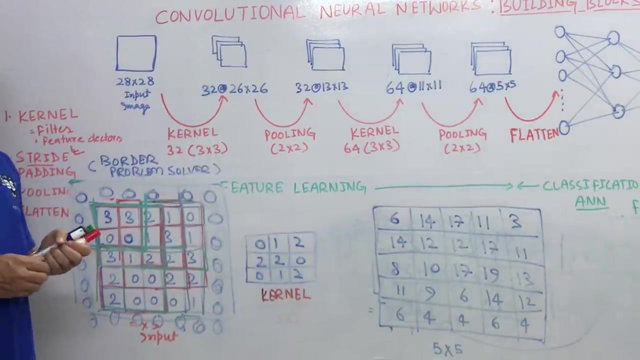 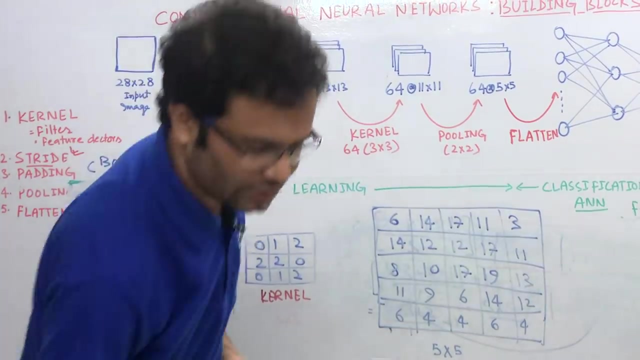 output: also 5 into 5.. So what we have to do, We have to add the one padding or the 4 side. The output of the padding, 5 by 5. this is the feature map matrix. Now I am going to use the pooling. So in the pooling we have the two concepts: one: 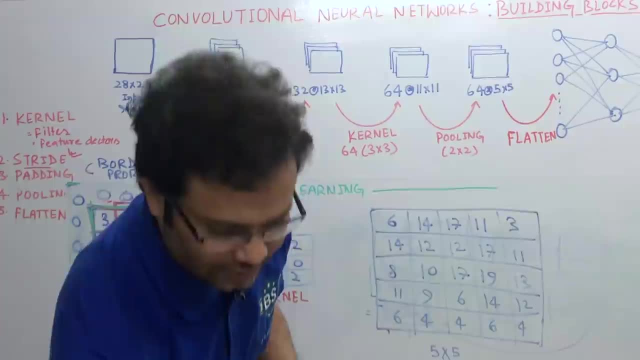 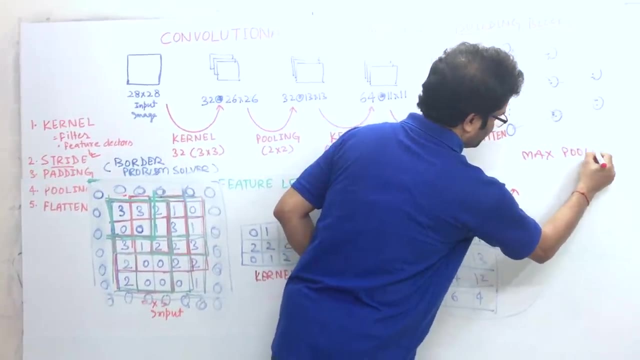 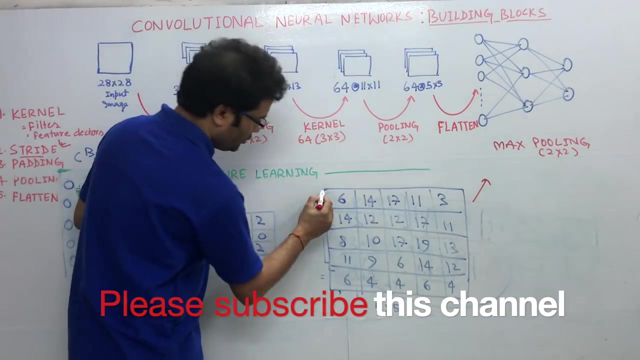 is the max pooling and one is the average pooling. So first go for the max pooling. So how it works If you take the max pooling 2 by 2.. So it is a 2 by 2 right? So 2 by 2 is this one. 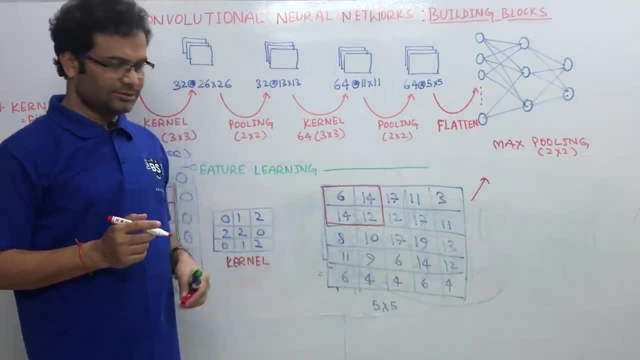 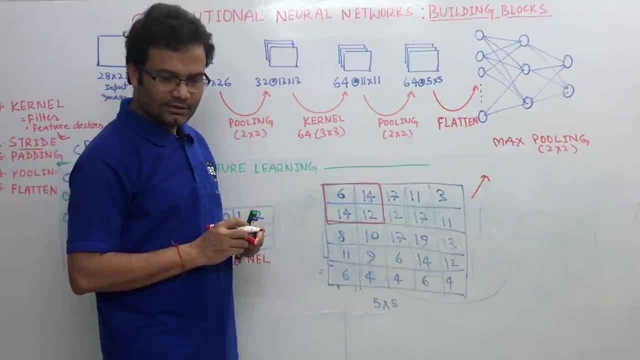 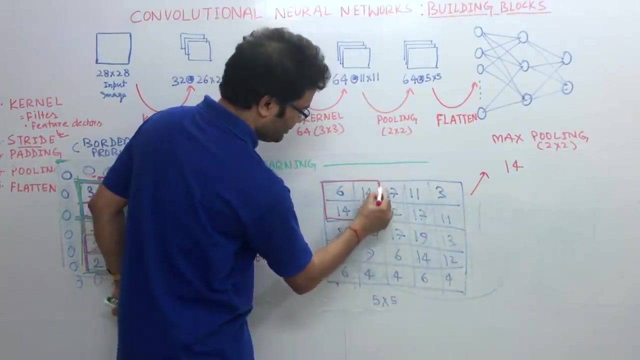 and it is saying max, So choose max out of these four. What is the max? Max is 14, right? So yes, max is 14, right. So take the 14. Here, what is the max? 2 by 2.. So 2 by 2. 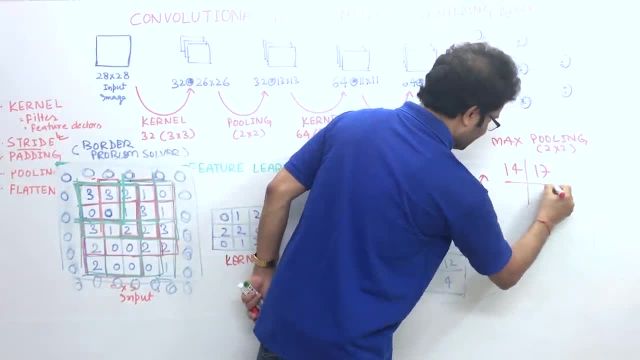 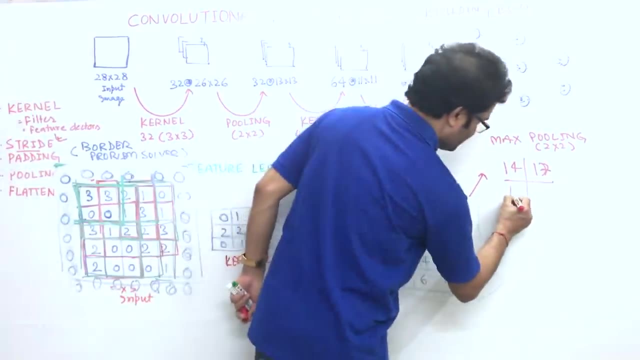 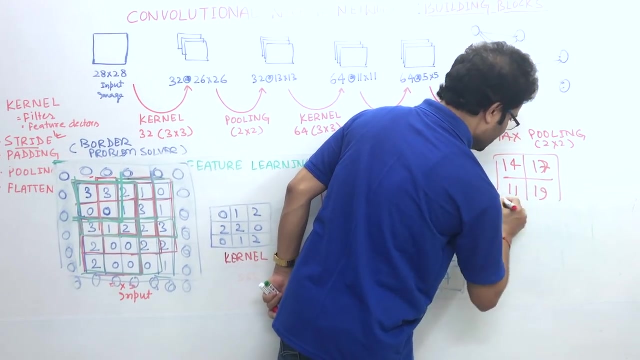 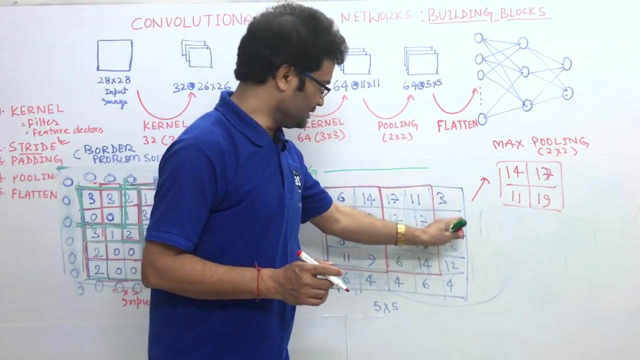 max is 17.. So take the 17.. What is the max here? 11, and what is the max here? 19.. So this is the output. if you apply the max column on this matrix- and we cannot consider this one because we do not have the 2 by 2 right- This is the max pooling. Now the max pooling. 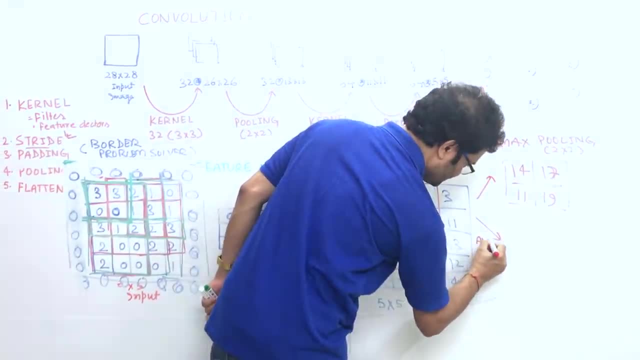 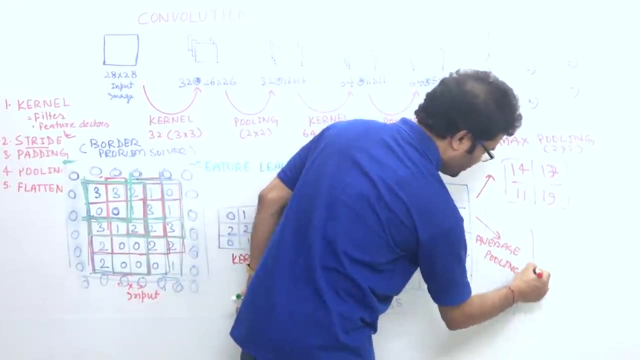 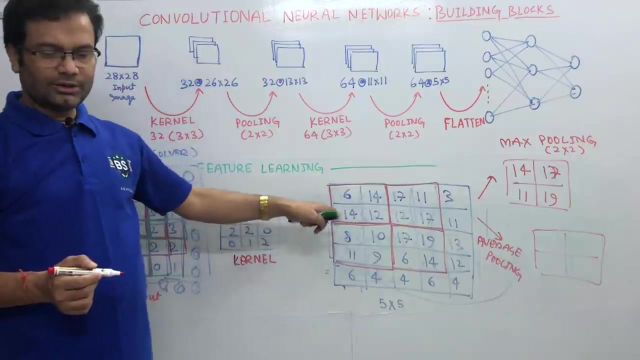 If you take the average pooling. so what you have to do, You make the average of 6, 14, 14, 2, so 6, 14, 14, 2, it will become 46. and take the. 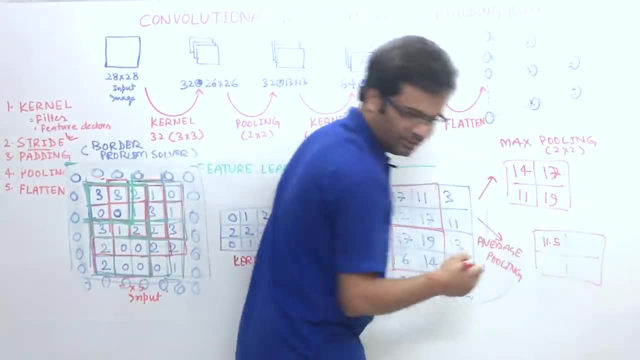 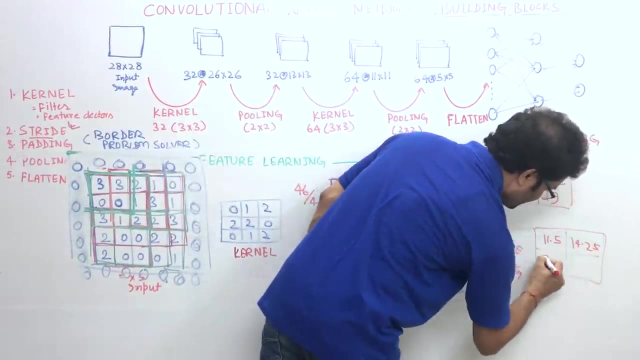 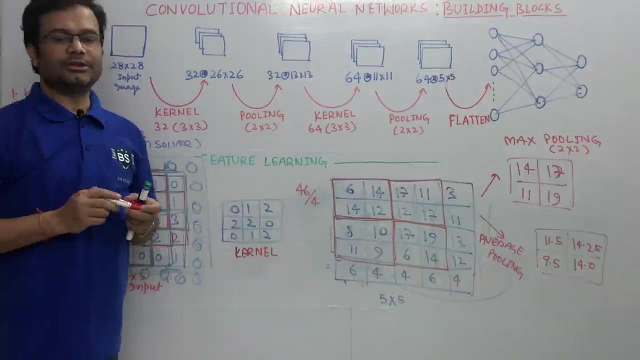 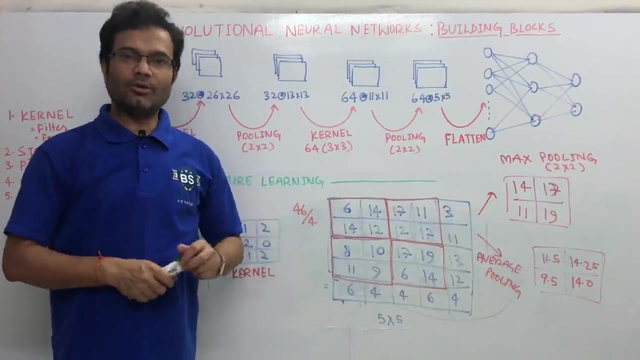 4, it become the 11.5, and this is the 14.25,, 19.5 and the 14.0,. so why use the pooling? The concept for the pooling is to reduce the dimension but with provided preserve all. 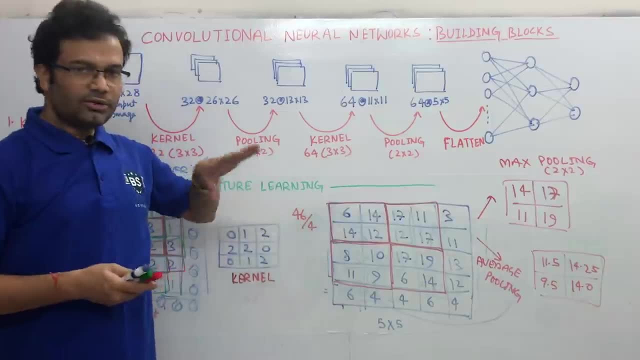 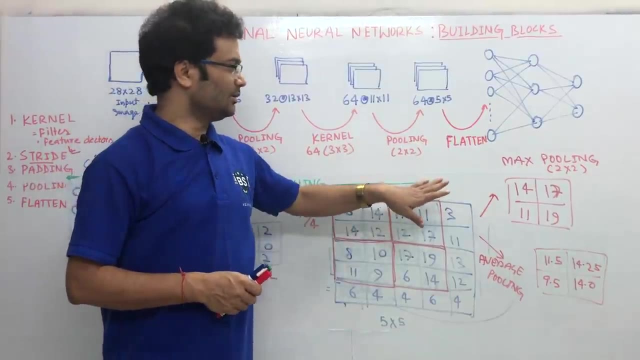 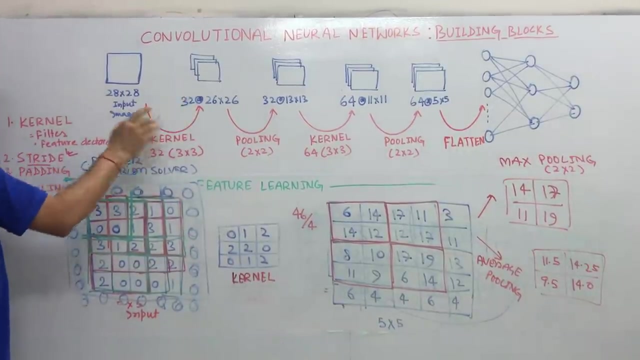 the important features. without using the all the important features, We can reduce the dimensionality. that is why max, that is why pooling we will use here right Now. if you done all those things, now I am quick, I am going to here and say now, if 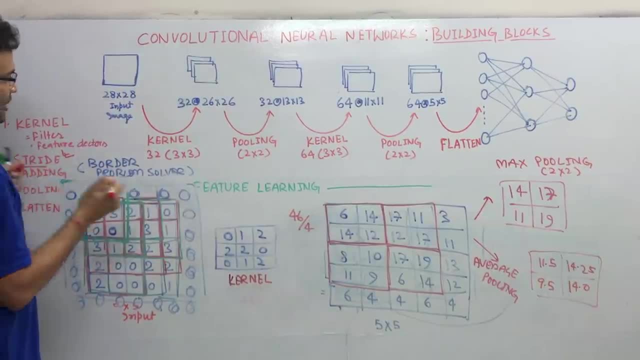 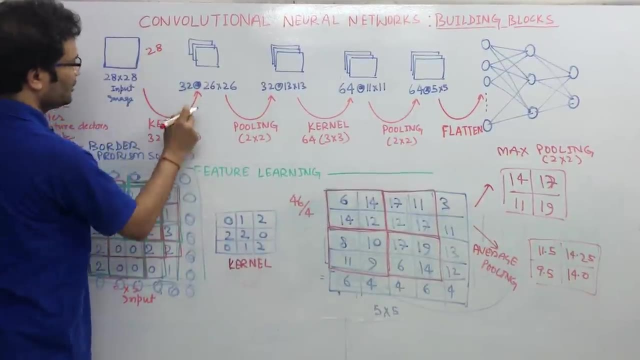 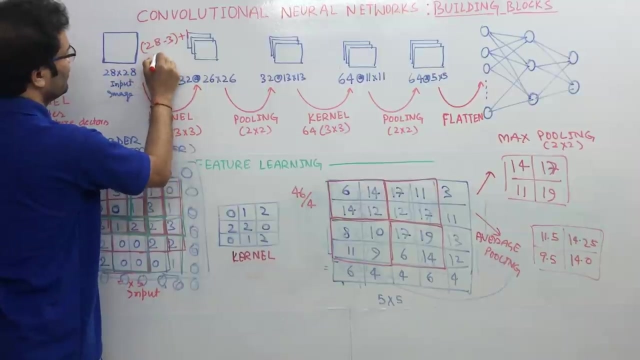 it is a 28 by 28 and the kernel is 3, how it become 26?? So we can see. first we can see here 28 minus 3 and plus 1.. So if you see 26.. 5 plus 1, 26,. so that is why we got the 26.. 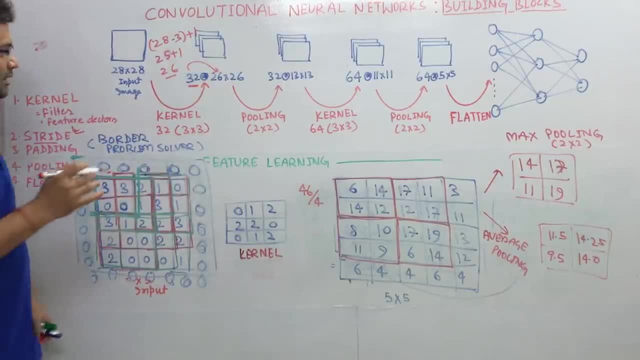 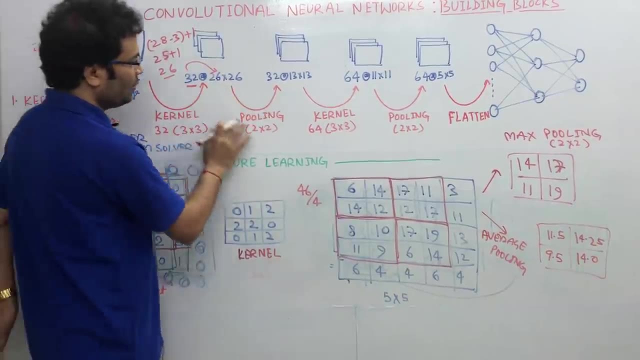 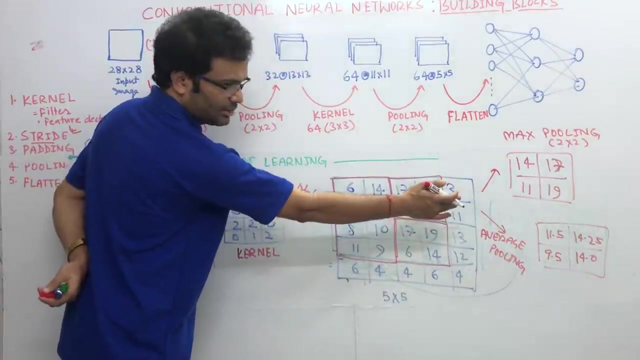 This 32 means I am taking the filter 32 filter to capture the more informations. that is not come in the picture. 32 will be the constant. Now I am going to pooling: use: use 2 by 2.. So what happen? if you see, here I had the 5, it become the 2 by 2, why? because 5 by 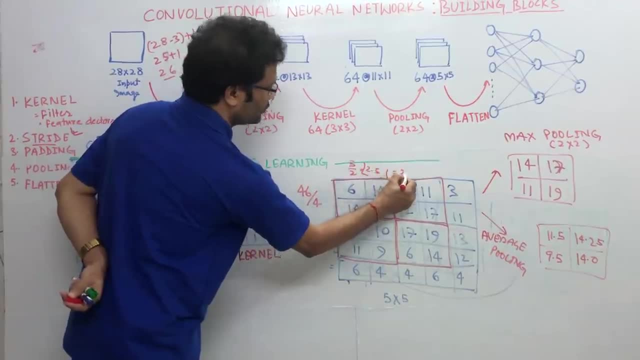 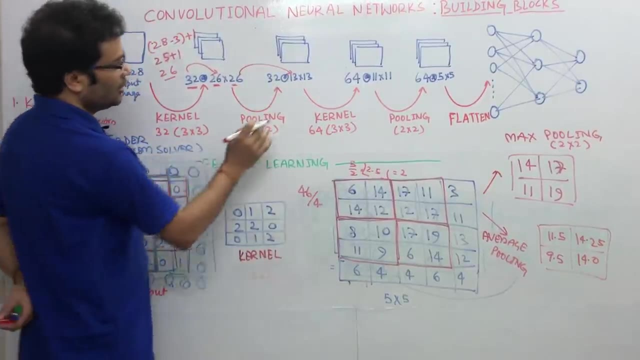 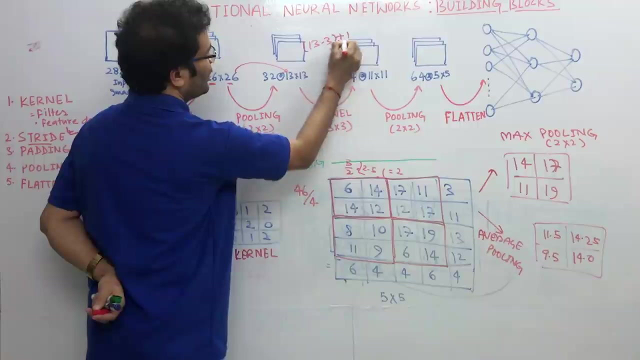 2, 2 into 5. take the floor, so 2.. The same way it become the half, 26, become the 13 due to this pooling right Now in this, take the kernel 3, what if you do 13 minus 3 plus 1 become 11.. 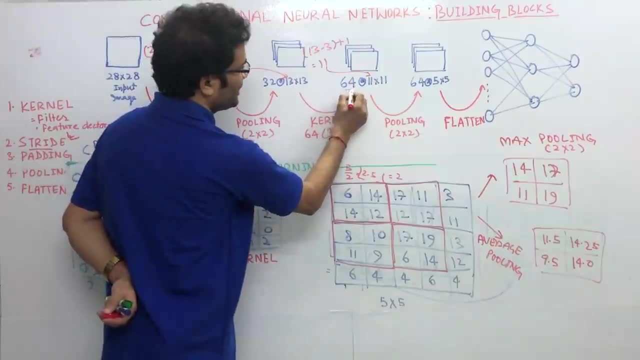 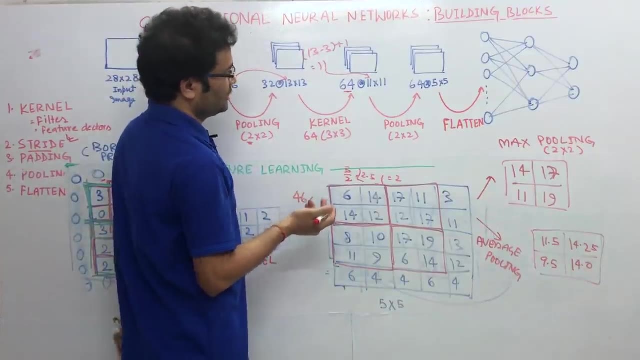 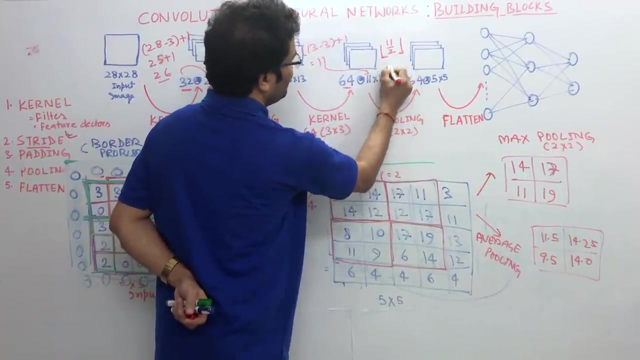 So, you see, become 11,. this here I am taking the 64 filter. we can take it right- depend upon the requirement of the research development things. Now, here we are going, the pooling. So 11 by 2, make the floor, it become the 5, so you can see the 5, right. 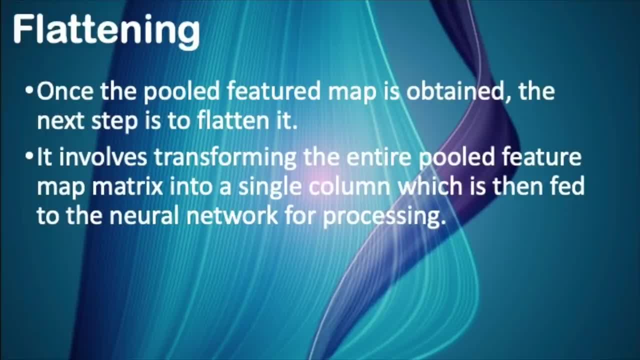 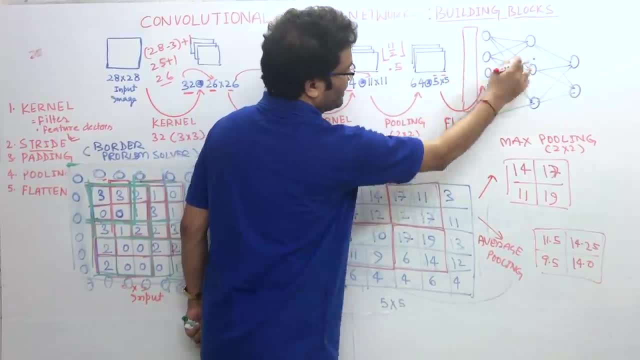 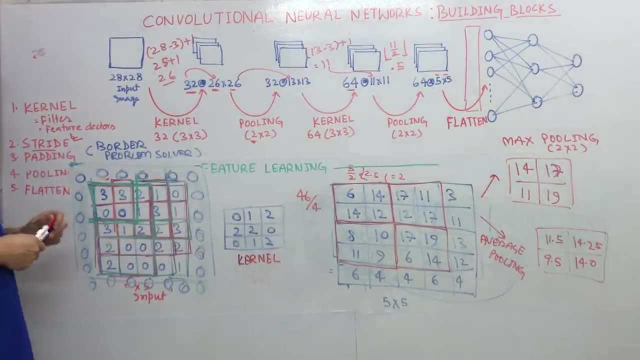 So now we have the 64 into 5 into 5, those we go make the complete one-dimensional array and that we go for the classification for reconnected network, How it works, all those concepts in the next video I will explain everything through the. 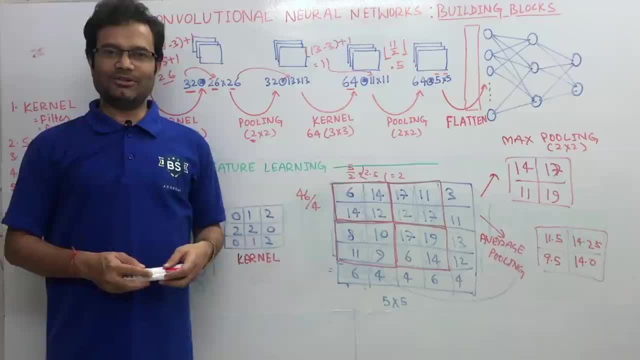 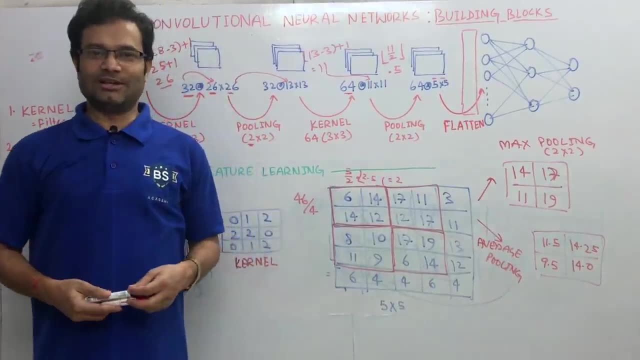 code so you can get the better understanding. So one request: please don't forget to subscribe the channel. I am putting more videos on the data science and the other new technology in very easy way. please click the subscribe button and don't forget to like the button. 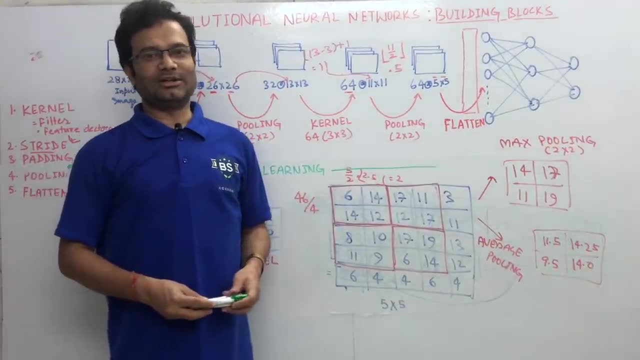 If you have any questions, use the comment box. I am active to giving all the answers immediate.